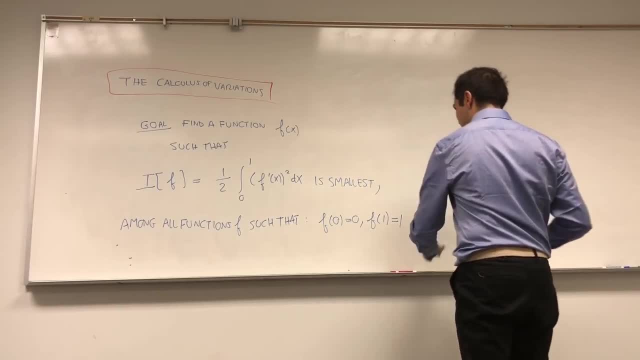 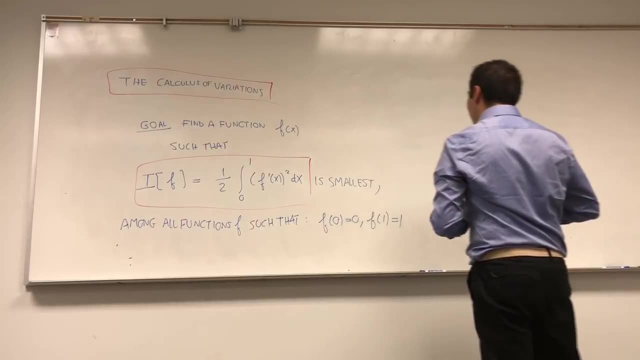 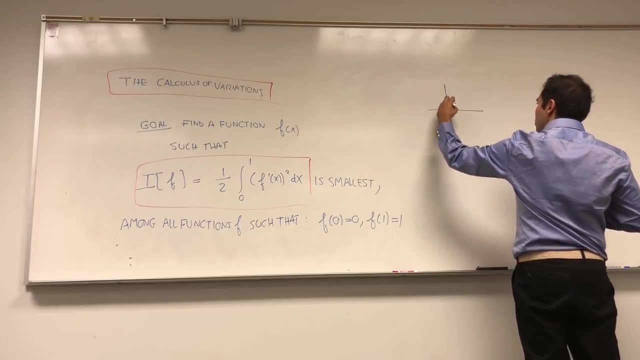 of one equals to one. In other words, you want to do the following: Among any function, f again smooth, you know, not even differentiable, almost It's almost everywhere with work, and f of zero is zero and f of one is one. so think, 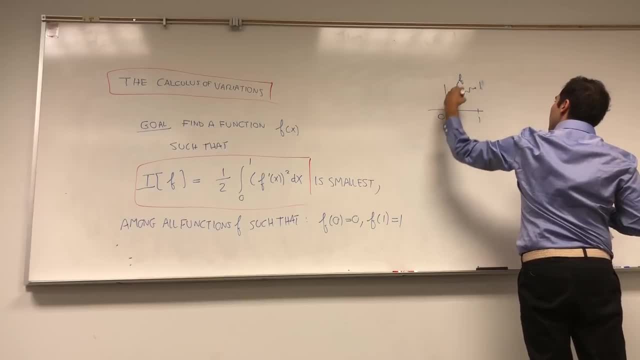 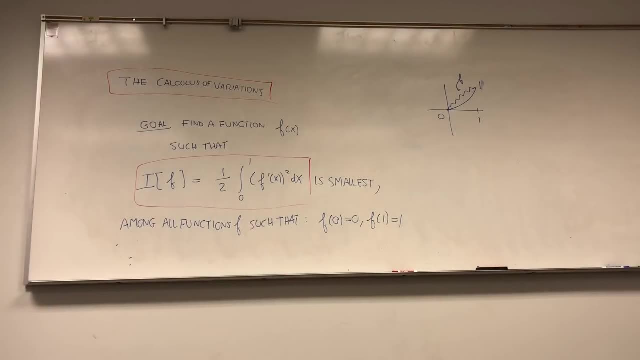 of a squiggly thing here, or maybe a parabola, or even the straight line, et cetera, et cetera. Among all those functions, you want to find the one or the ones for which this energy. 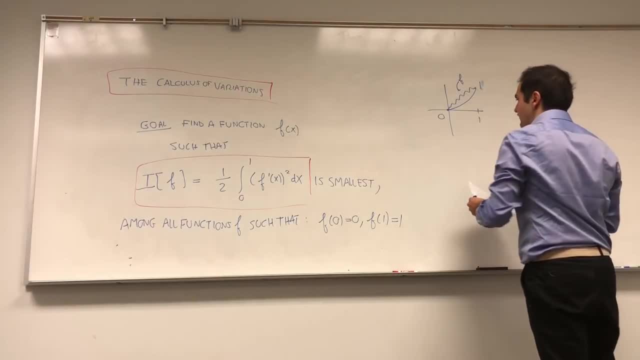 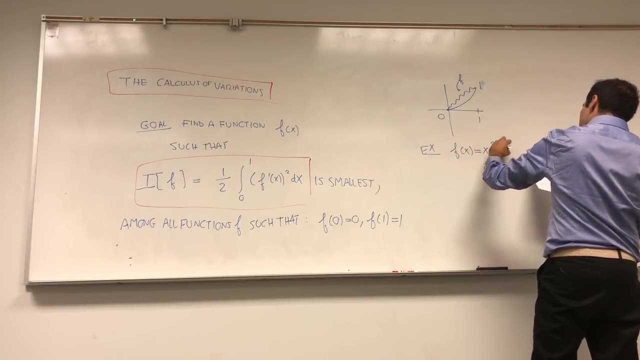 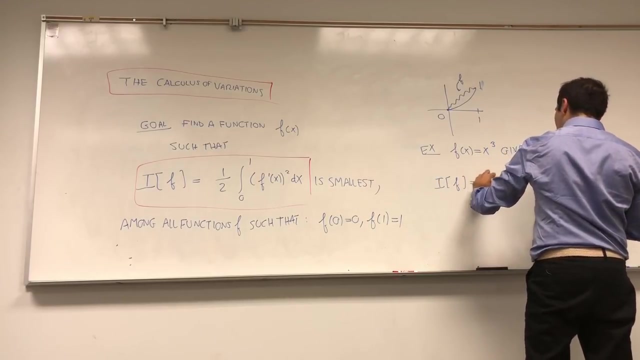 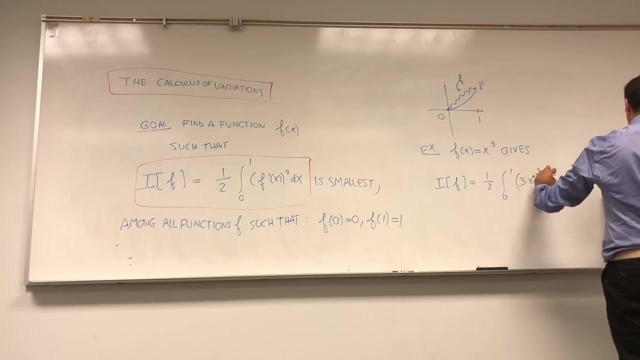 is the smallest. Okay. So for example- let me just give you a couple of examples- f of x equals to x. cubed gives the following thing: i of f is integral, so one-half integral, from zero to one derivative squared, so three x squared squared dx, which is one-half integral. 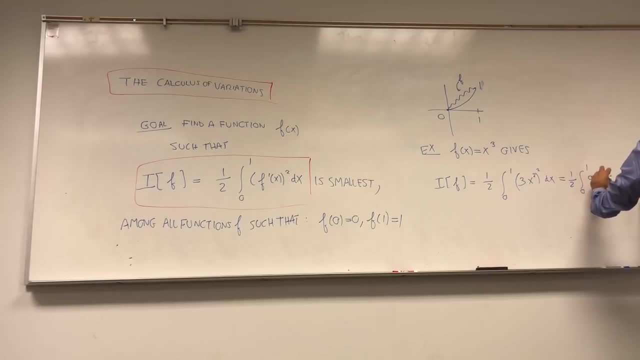 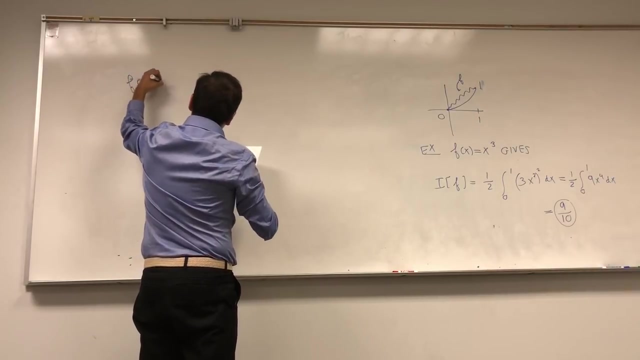 from zero to one of nine. x to nine, Okay, x to the fourth, dx, which is so nine-halves over five, so nine-tenths, because the antiderivative is nine. x to the fifth over five, So the energy of this function is nine-tenths. f of x equals to x squared, then i of f equals. 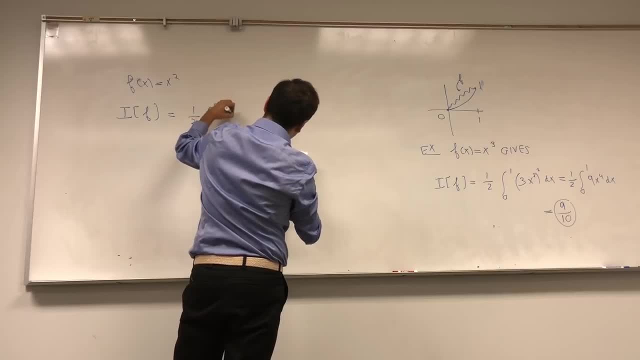 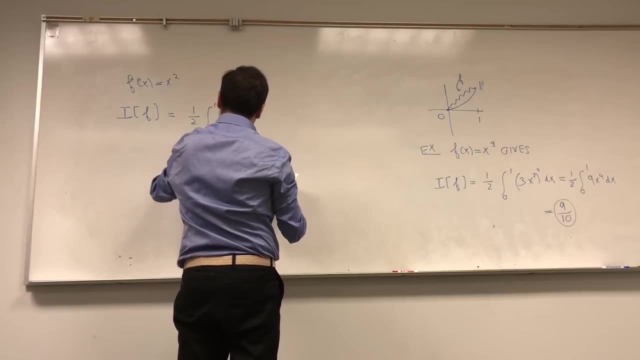 to one-half integral from zero to one Integral from zero to one of two x squared dx, and that's one-half integral from zero to one of four x cubed dx, which is one-half times x to the fourth, which is one-half. 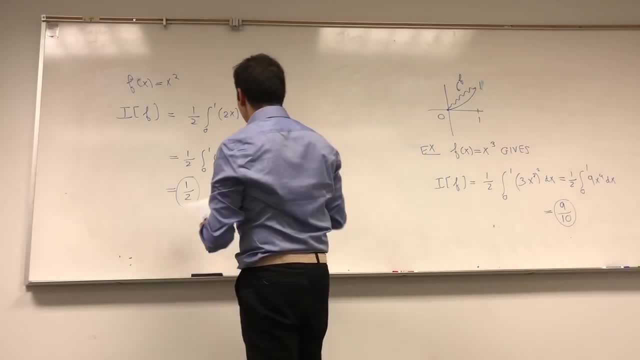 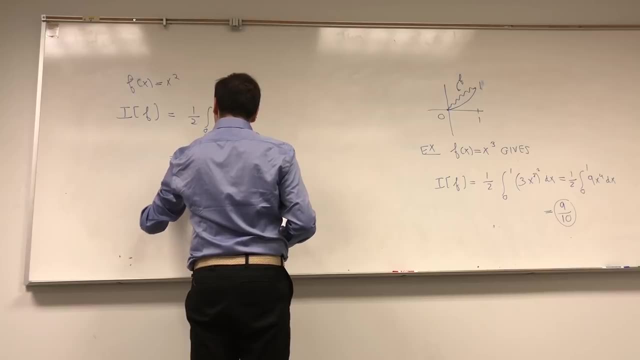 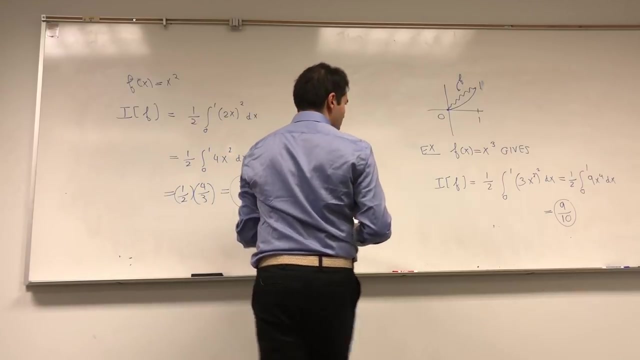 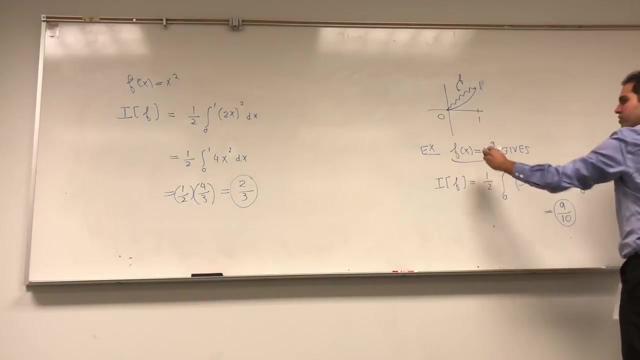 I'm sorry, I know It's four x squared, Okay, Okay. Okay, Four thirds. Okay, Sorry about that. One-half times four-thirds x cubed, so it gives you four-thirds, which is two-thirds. You can already see if you had to choose between the function x cubed and the function. 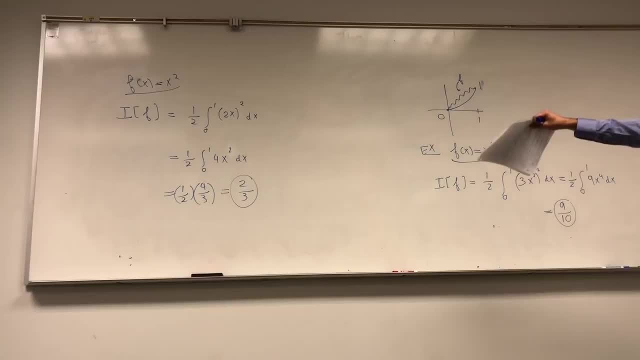 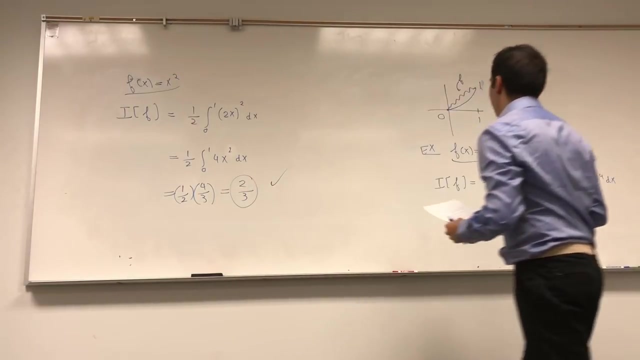 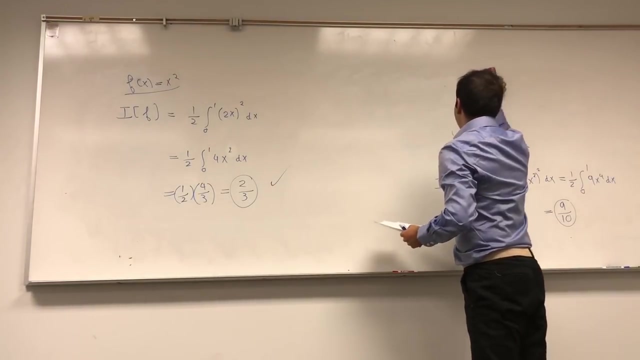 x squared, then x squared is a winner, because the energy it takes less energy to calculate i with x squared than to calculate i with x cubed. So this is a better thing, right? And if you think about it heuristically, the answer should make sense because sort 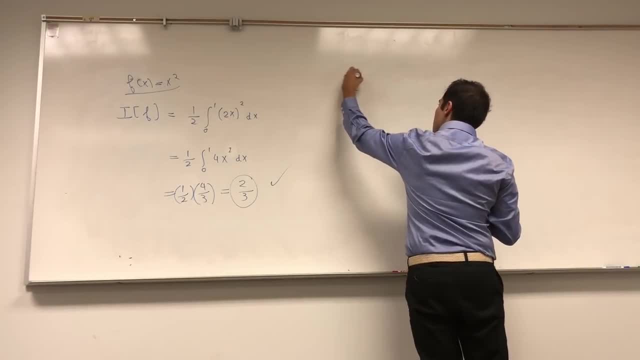 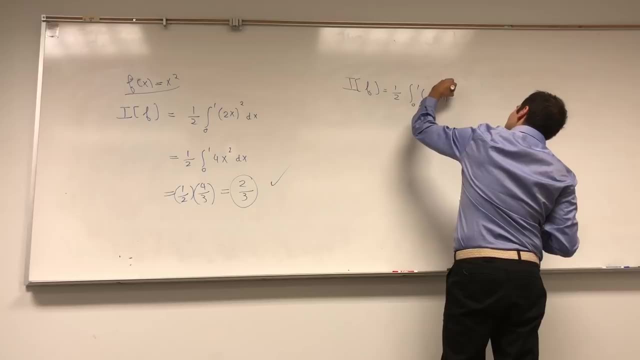 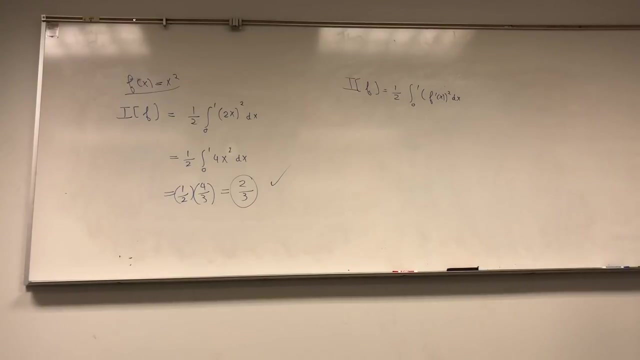 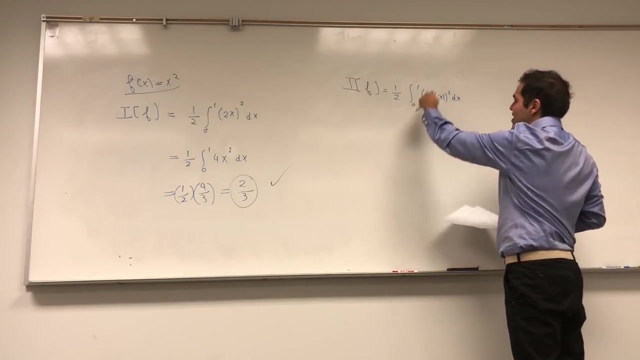 of. if you take i of f again, one-half integral from zero to one dx, and that's one-half integral from zero to one, One-half integral from zero to one of f, prime of x squared dx. So the smaller the derivative is, or the smaller it moves, the better, because if f changes, 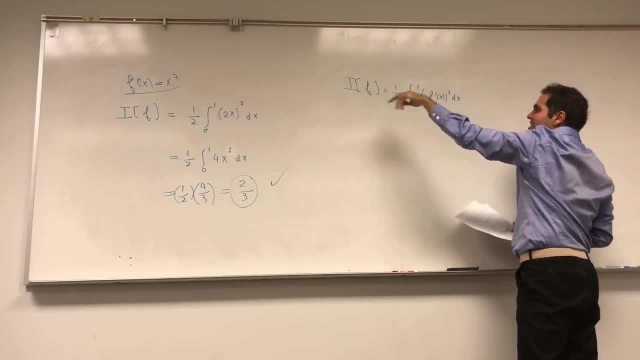 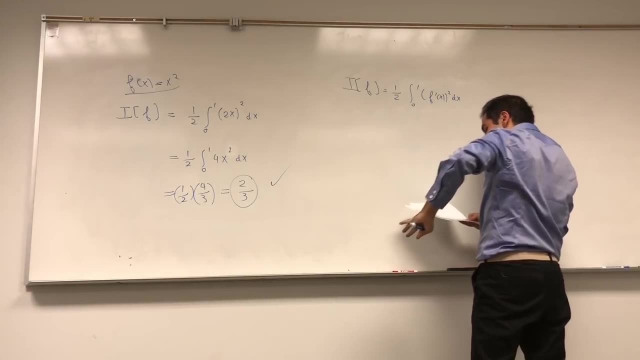 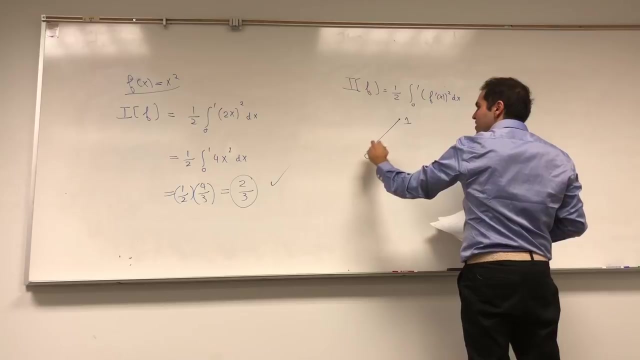 a lot. if it squiggles a lot, then the derivative squared becomes bigger and if you integrate that it's a problem. So, intuitively, the best choice is to integrate, Okay, Okay. So the solution should be the one that doesn't move as much, namely, intuitively, the minimizer. 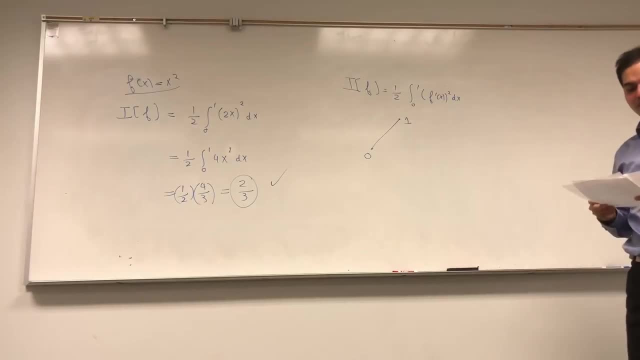 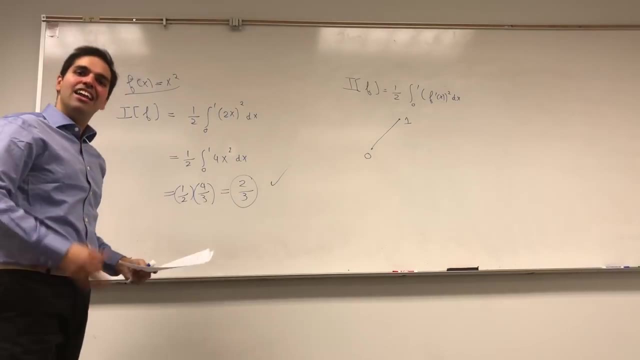 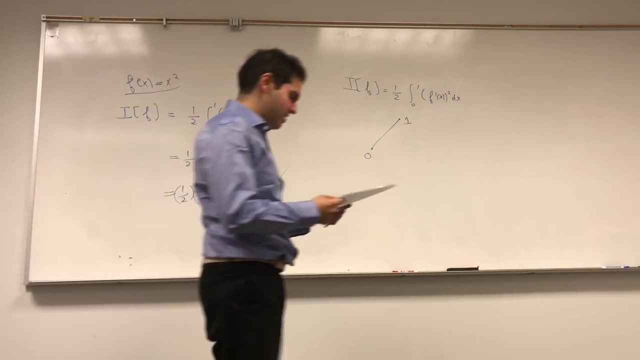 of this energy should be the line connecting zero and one, But of course we want to prove this and we'll do this very soon. Let me just give you a little fact that we'll need in a second, So maybe let's see. 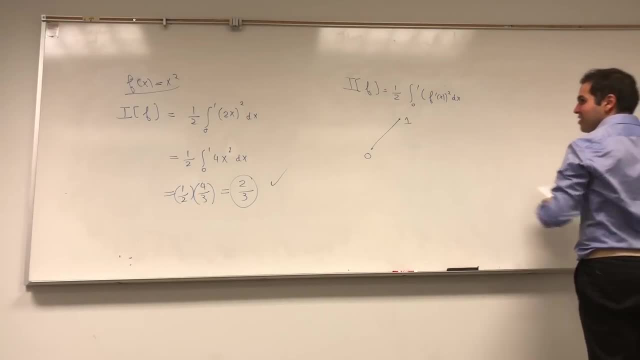 Let's see. Okay, So that was part one. So that was part zero, and now part one. Okay, Here's a little fact. Suppose you have a function g that is zero, at the endpoints zero and one and g looks. 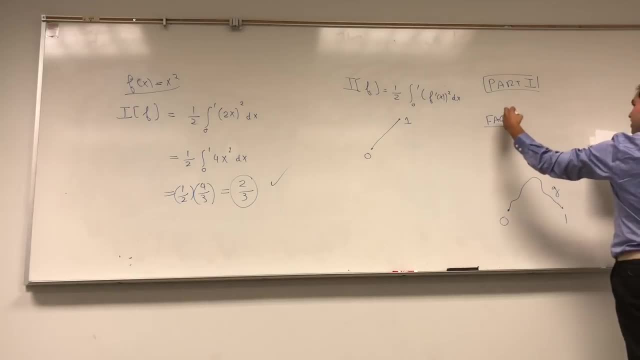 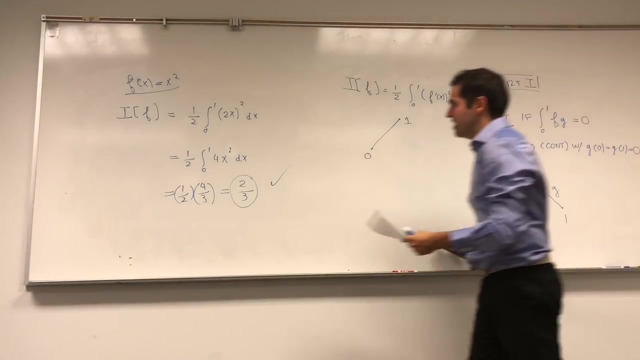 like that And suppose: if integral from zero to one, fg equals to zero for all g, Okay, Okay, So g again continues with g of zero equals to g, of one equals to zero. In other words, if you test f with any function g and you get zero, then f has to be identically. 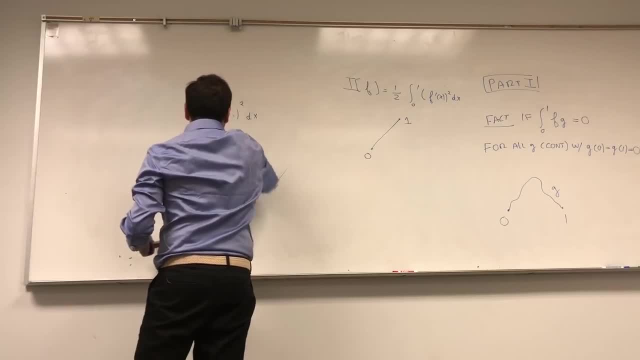 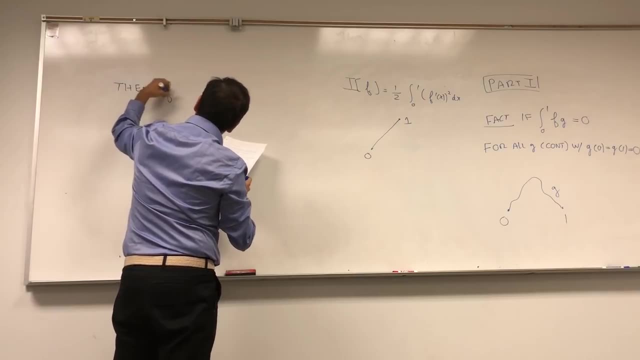 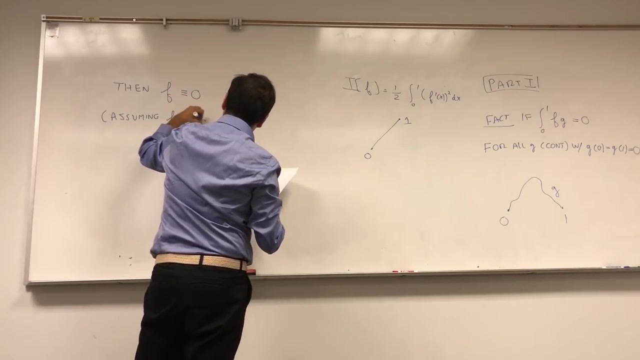 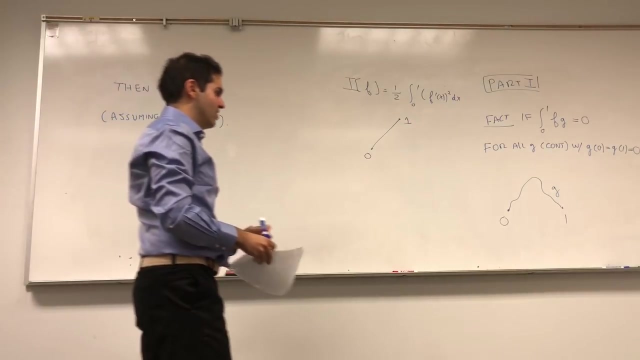 equal to zero. if it's continuous, Then f has to be identically equal to zero. Okay, Then f identically equal to zero, assuming f is continuous, And we will need this fact because we will essentially show that if you test our function. 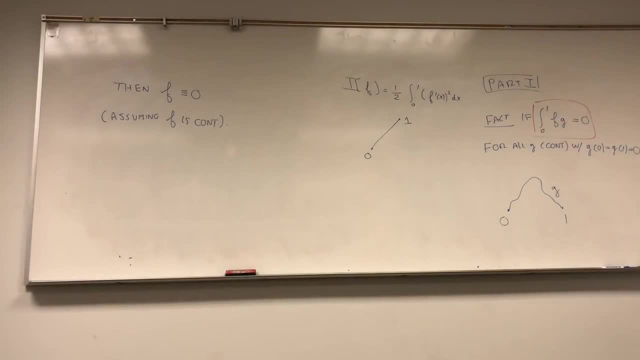 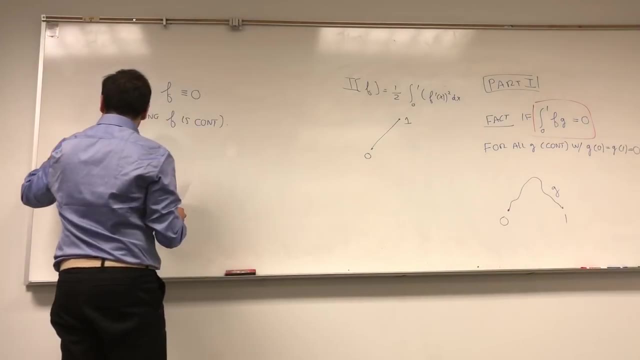 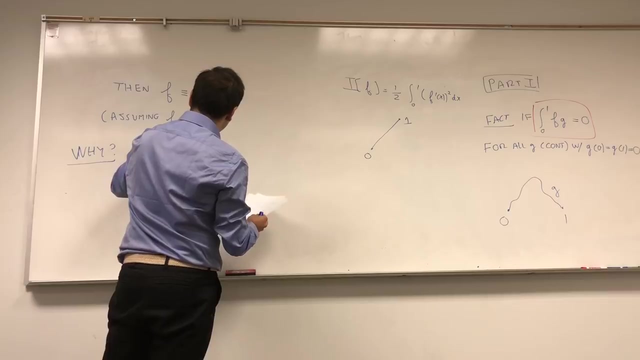 against a differential equation. you always get zero, so this function will be identically equal to zero. Let me quickly show that It's a very nice proof. Okay, So y suppose f is non-zero- zero for some x-naught. 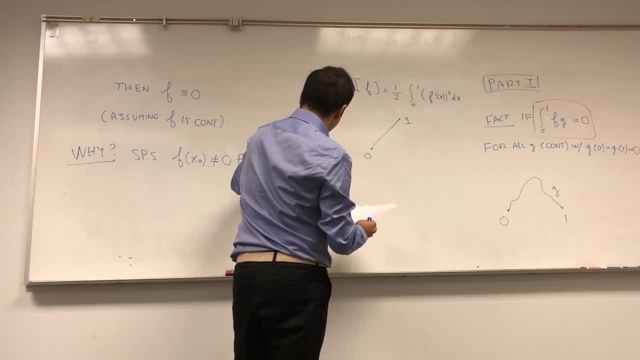 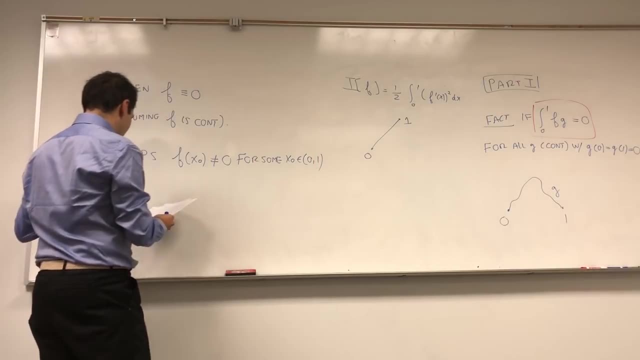 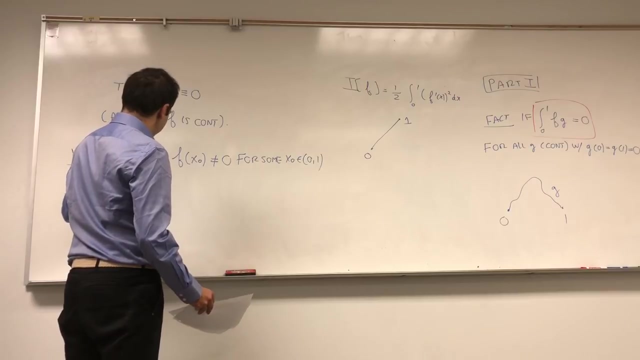 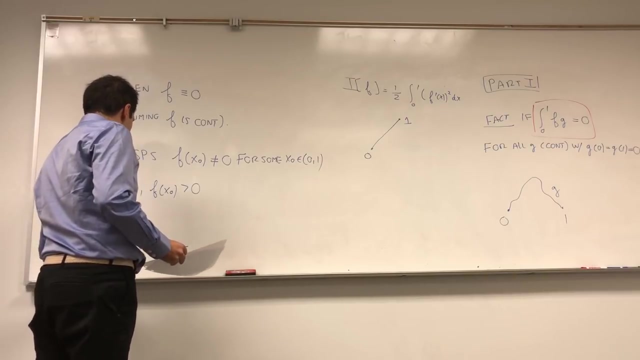 X-naught in the interval zero, comma one. I'll talk about the endpoints in a second. okay, Then if it's non-zero, it's either positive or negative. Assume it's positive, X-naught is positive. So we have this function here. this is zero, this is one, and we know f is positive here. 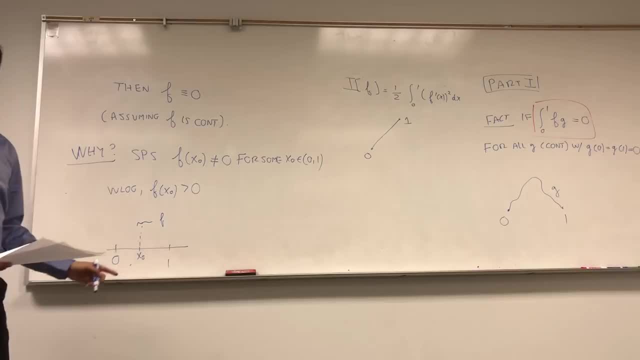 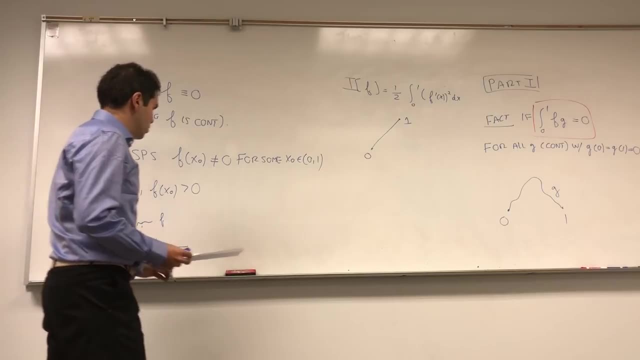 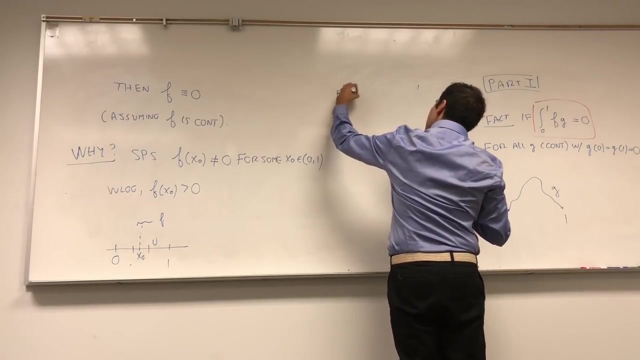 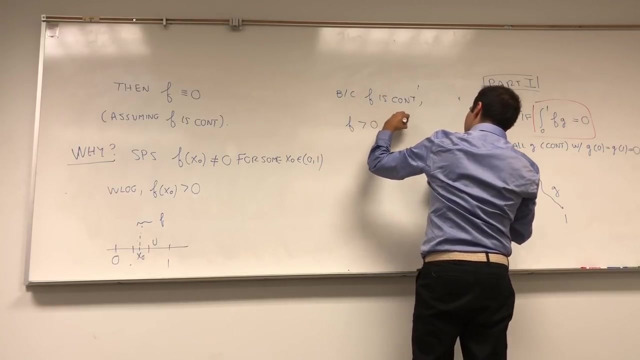 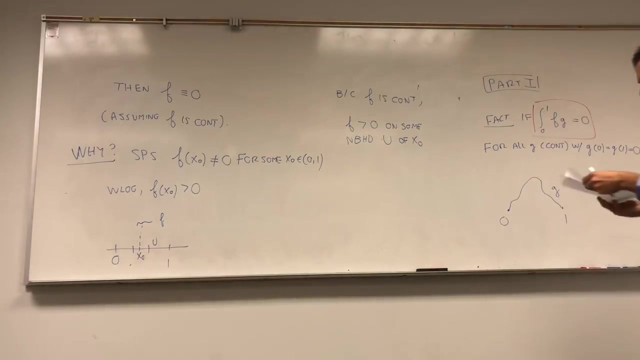 Well, because it's continuous, f also has to be positive in the neighborhood of x-naught, So maybe in the neighborhood u. So because f is continuous, continuous f is positive on some neighborhood NBHD of capital, U, of x-naught, all right. 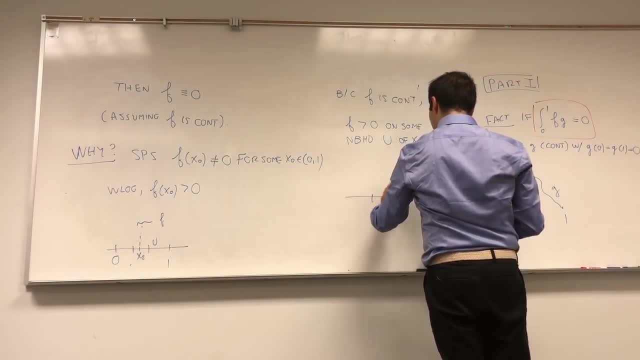 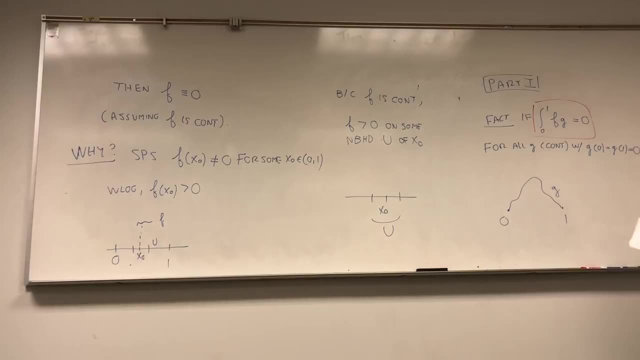 So again, we have this neighborhood u. That's x-naught. Okay, So we have x-naught where f is positive, and all you need to do is to define the following function, and you can do this using what's called bump functions. 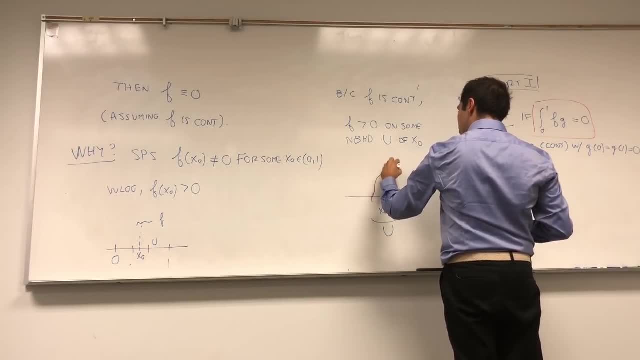 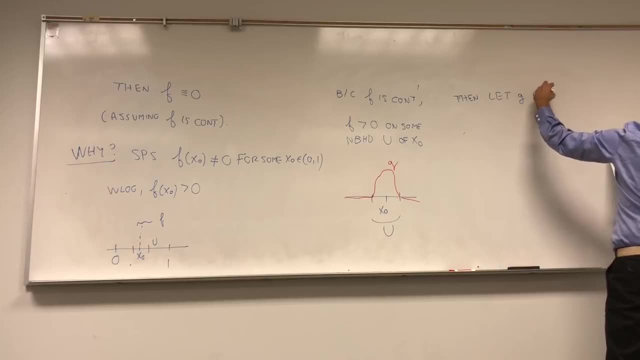 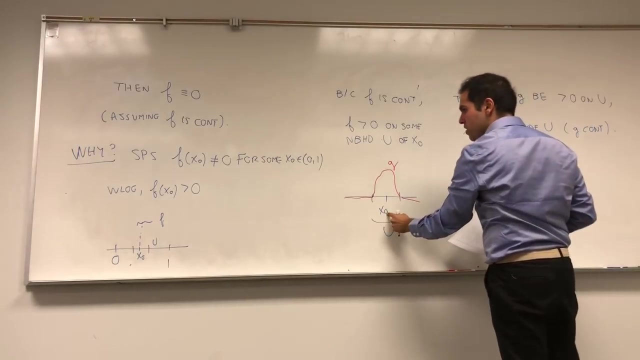 Define a function g that's just positive on u and everywhere else is negative. Let g be positive on u and zero outside u And g is continuous, In particular because you know where x-naught is inside the interval zero comma one g has. 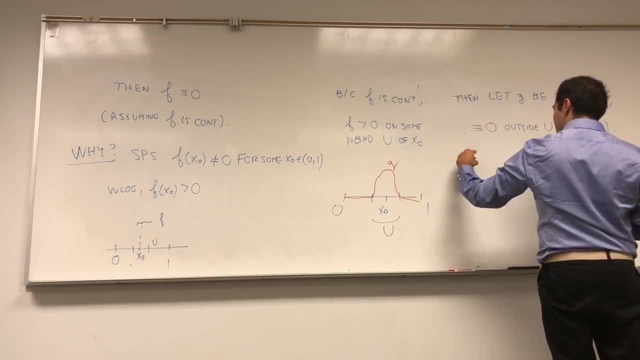 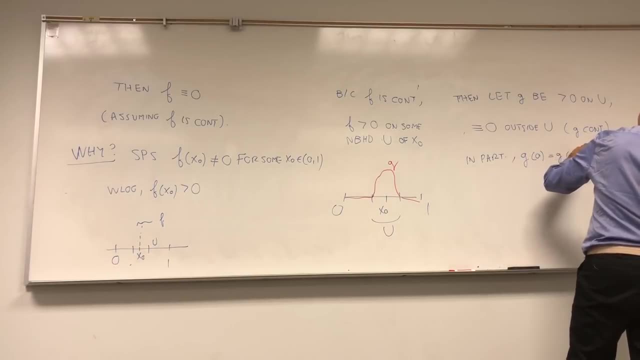 to be zero, at the end points zero and one In particular, g, of zero equals to g, of one equals to zero. So g is a very good test function that we can use. Okay, So, on the one hand, because g satisfies those properties we know by assumption, it equals. 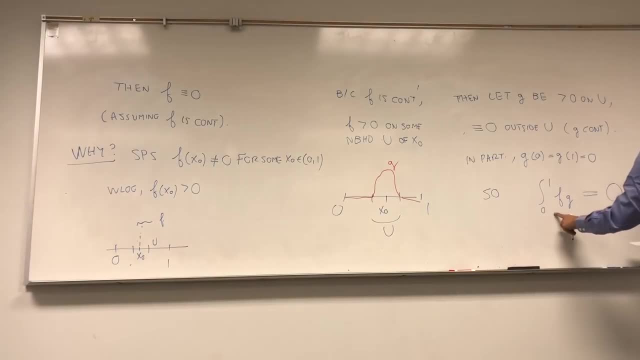 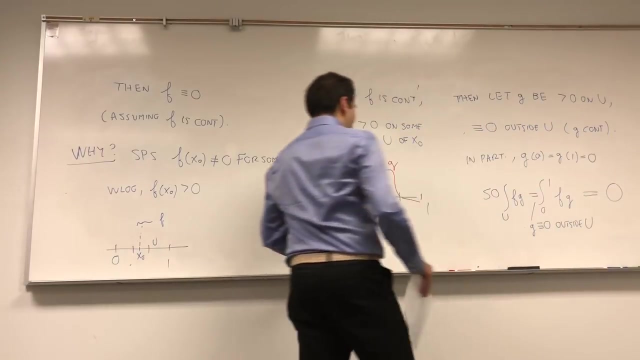 to zero. On the other hand, because g is zero outside of u, this integral is equal to the integral of u of fg. okay, G is identically equal to zero outside u. So the party happens in u. Okay, It's a cool neighborhood, but what do we know about u? 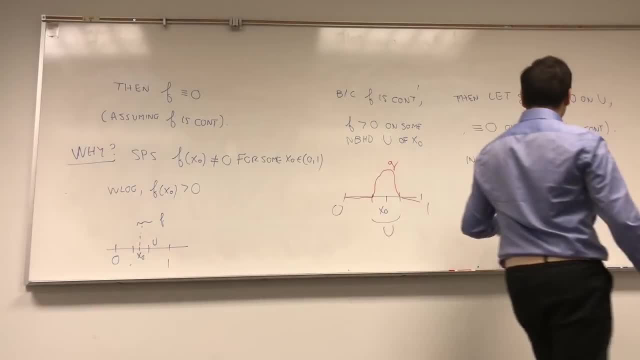 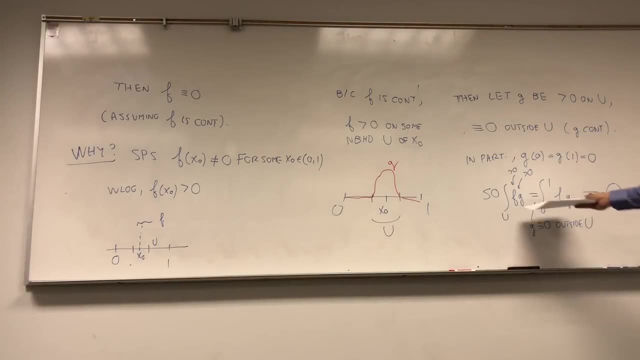 We know that f is positive in u and also g is positive in u. So this is the integral of a positive function which is positive, and I'm positive about that. So what do you get? You get that zero equals to a positive number, and that's a contradiction, at least in the 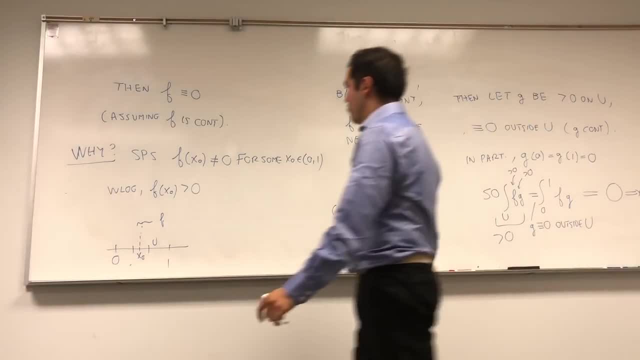 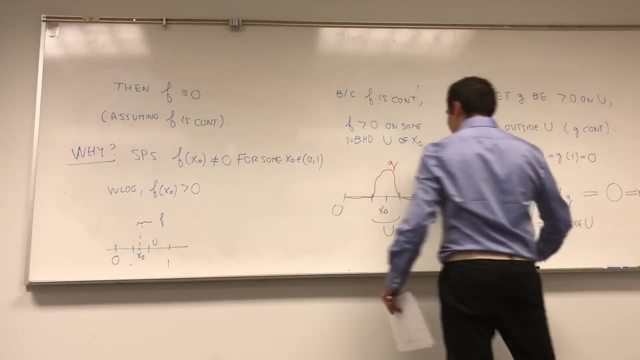 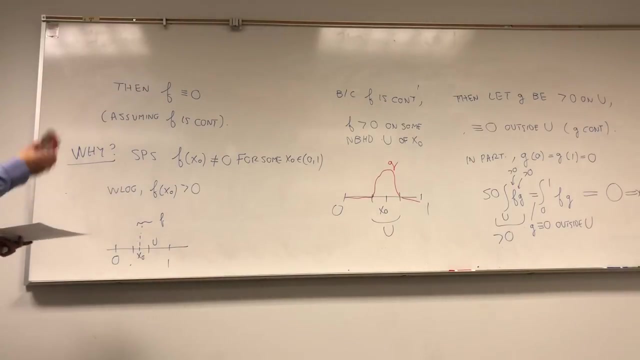 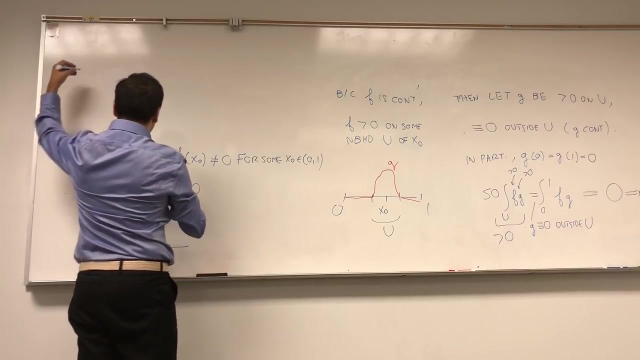 world. A contradiction with what? A contradiction with the fact that f is non-zero at a point. So f is identically equal to zero on the open interval, zero comma one. but what about the end points? It's actually just follows from continuity. 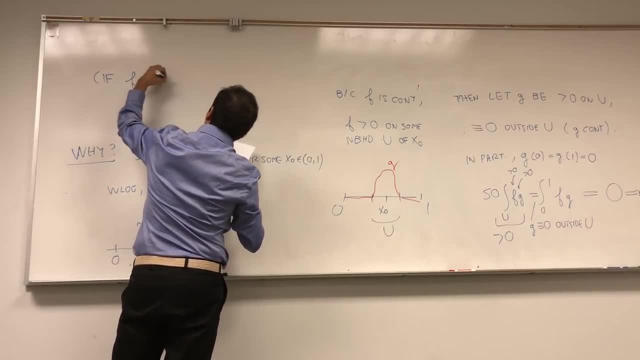 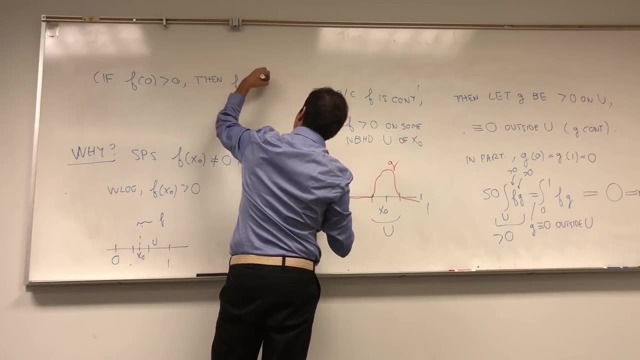 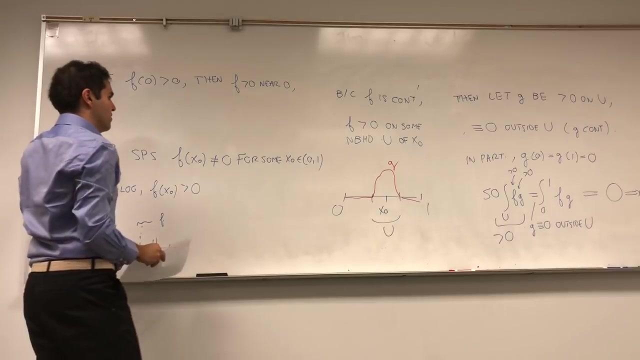 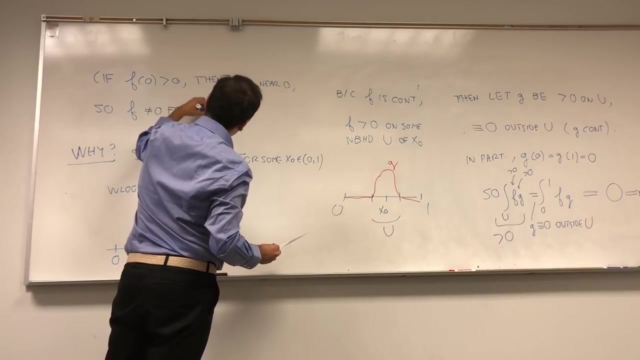 So if let's say f of zero is positive, Then Right, Because f is continuous, f is positive near zero. So in particular, f is still non-zero from some point near zero. So f is non-zero for some, x zero near zero. 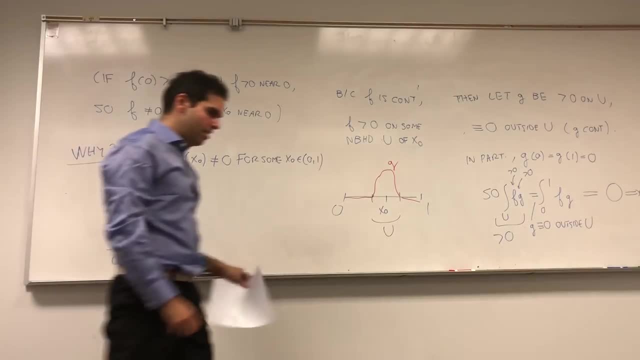 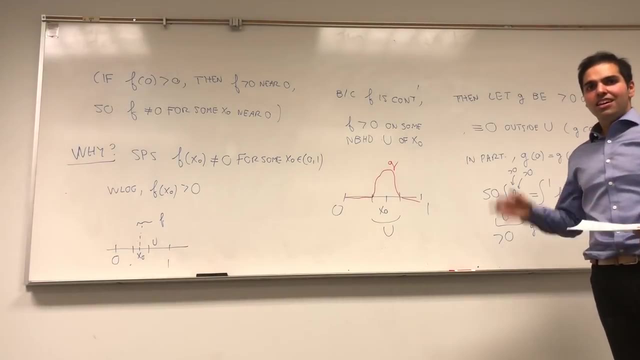 And you can still use the same proof. Okay, Very good. And that was to illustrate this technical fact that if you test a function against some other function, g and you get that it's always zero, then the original function has to be the zero function. 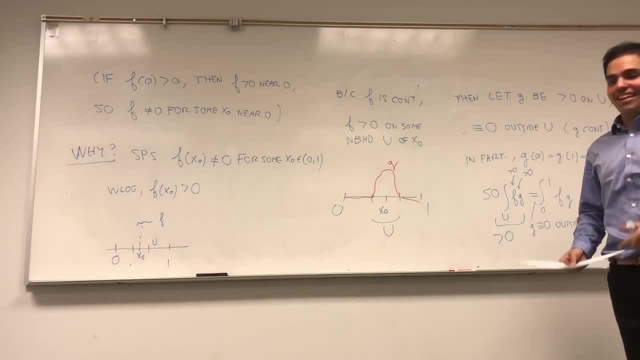 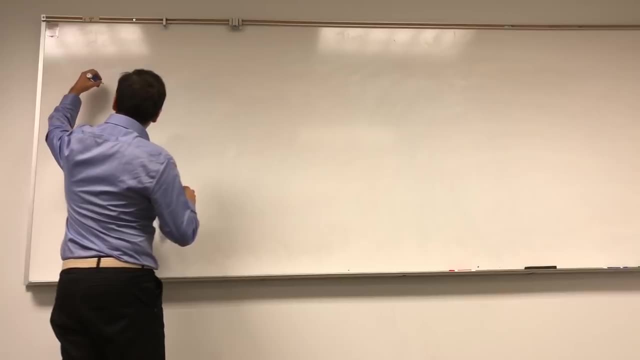 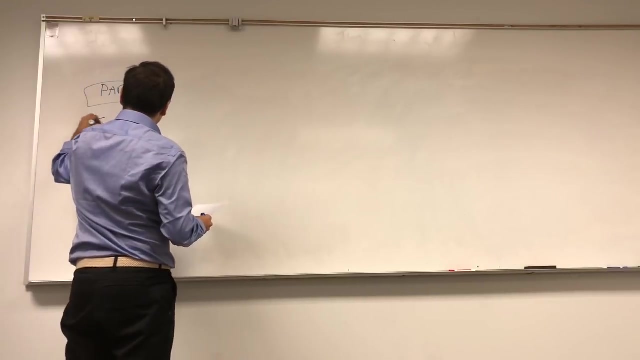 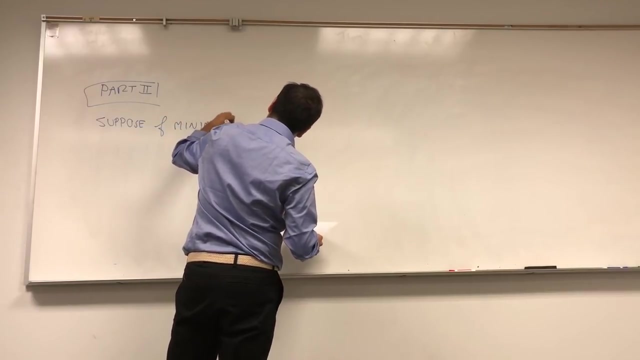 And this will be useful in a second. Okay, Now we can play, Spielen wir? Okay, Because we can now solve our problem at the beginning. So part two: Okay, Suppose f minimizes this functional So i of f, which is one half integral from zero to one f, prime of x squared dx. 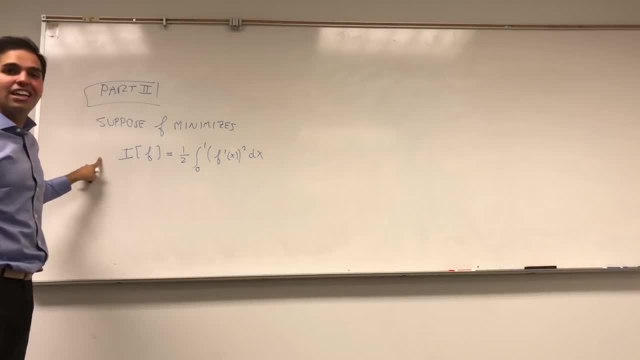 Our goal is. here's our game plan: we want to find a differential equation that f has to solve And we want to solve that differential equation. That's why I always said this relates to the, to partial differential equations. So now let g be arbitrary, and you'll see why I say that. 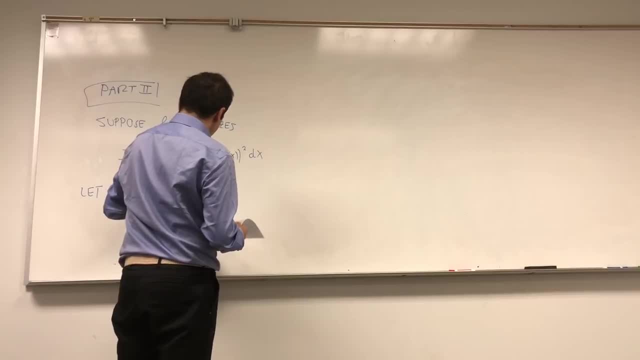 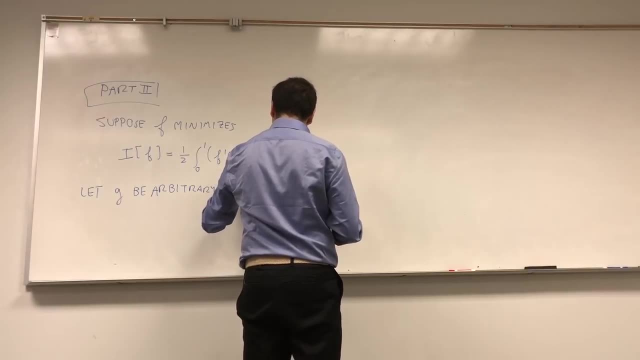 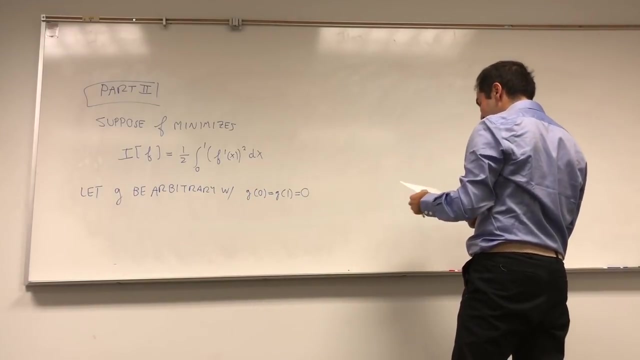 Let g be arbitrary against smooth and arbitrary with you know, is g zero at the end points. g of one equals zero. Okay, g of one equals zero, And you'll see in a second why this is true. And consider now the following. 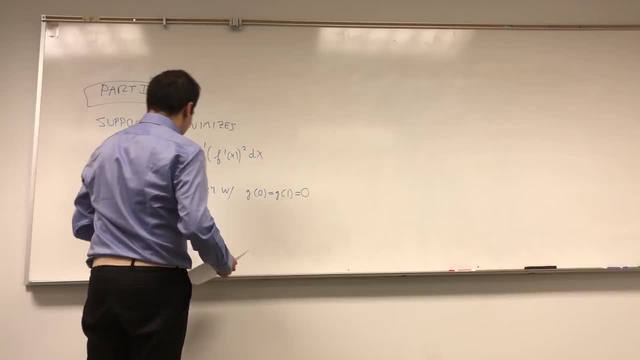 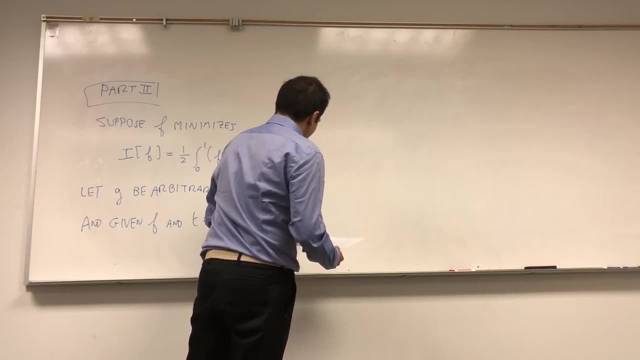 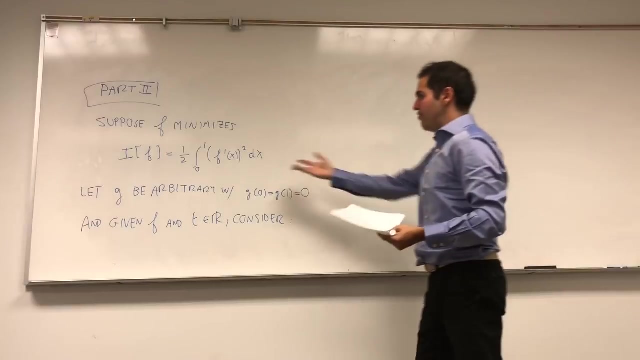 And given f and let's say some real number, t, consider the following function. And before I write this down, I want to tell you something. This is a difficult problem, All right, Because among all the functions, you want to minimize this thing. 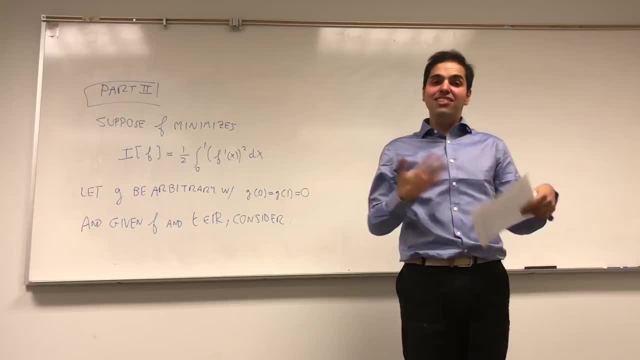 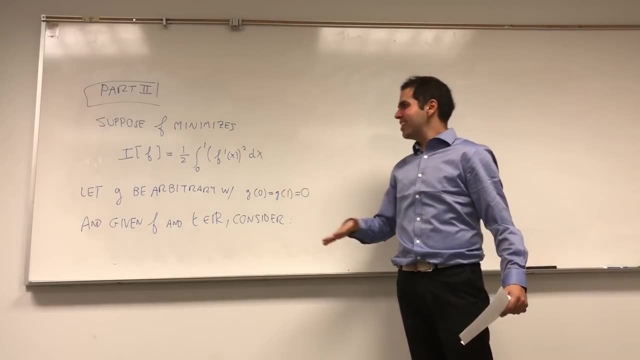 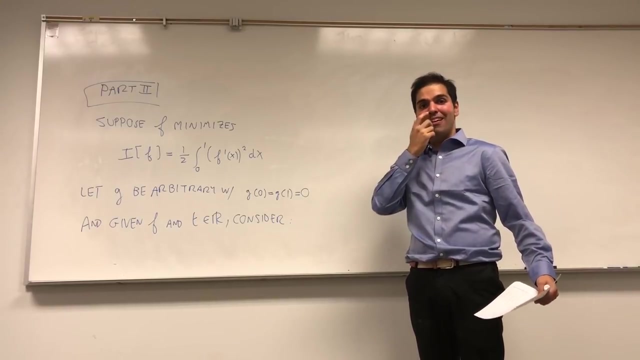 So it's really a problem about functions And it's very hard to do calculus on function spaces. But here's the cool thing about this: We will take this difficult problem and turn it into a one-dimensional calculus problem, Which is why this problem is called the calculus of variations. 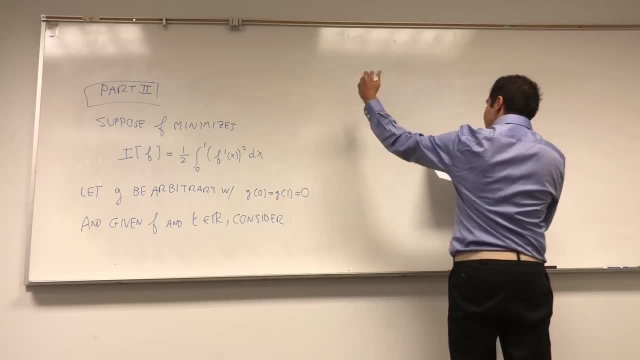 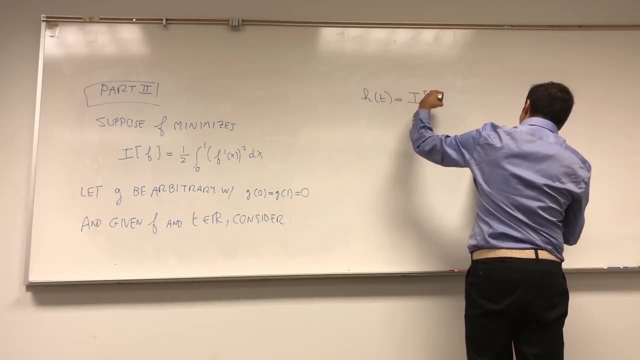 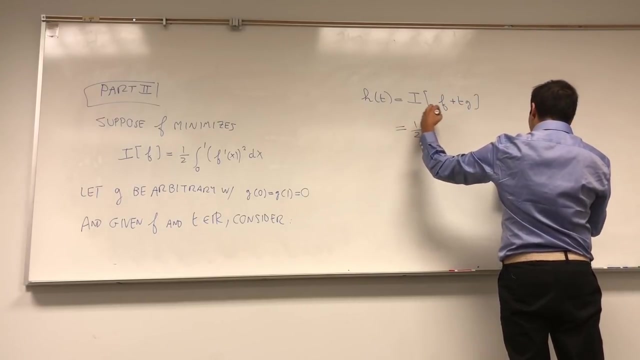 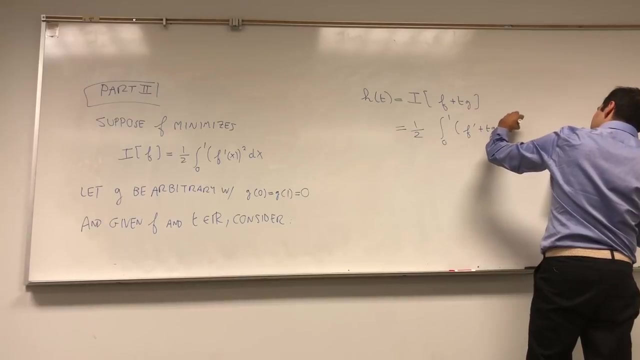 Because If you have f and t, Okay, Consider the following single variable function, h of t, which is the energy of f plus tg, okay, Which is, if you want, one half of the integral of f prime plus tg prime squared dx. 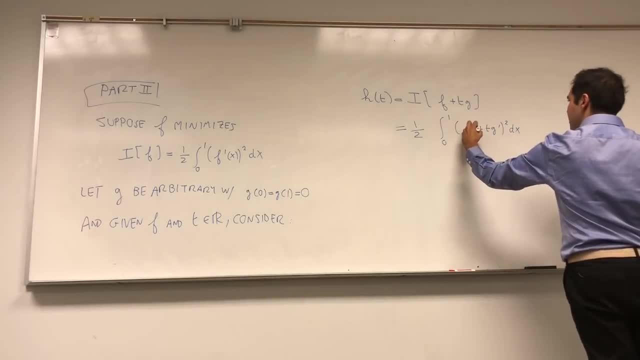 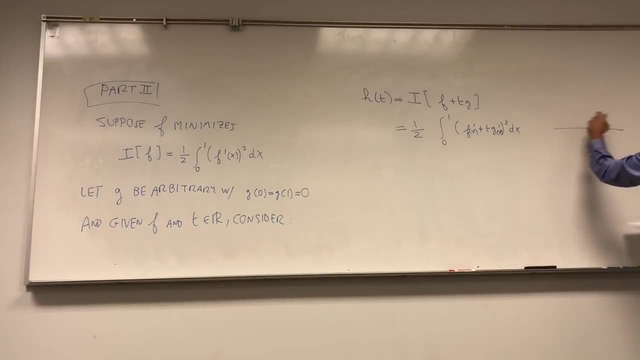 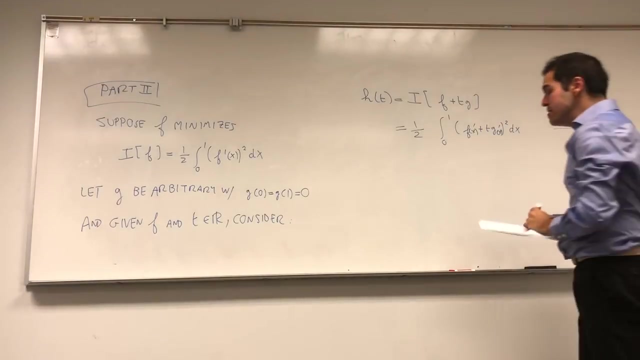 Again, not dt, but t is a parameter, if you want. Okay, Okay, Okay, Okay. And let's also look at this picture. So this is t, This is zero. We know that f minimizes this thing, Right. 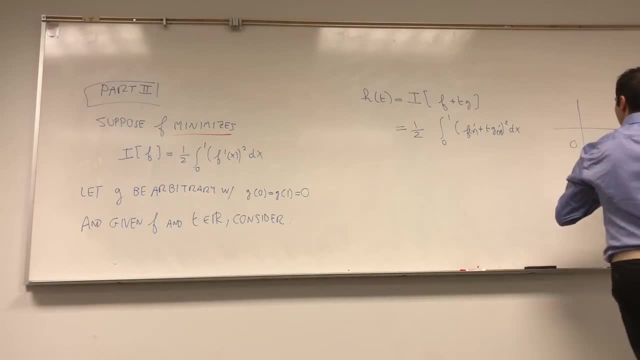 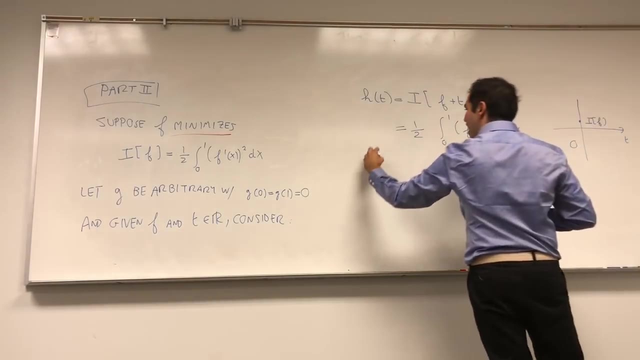 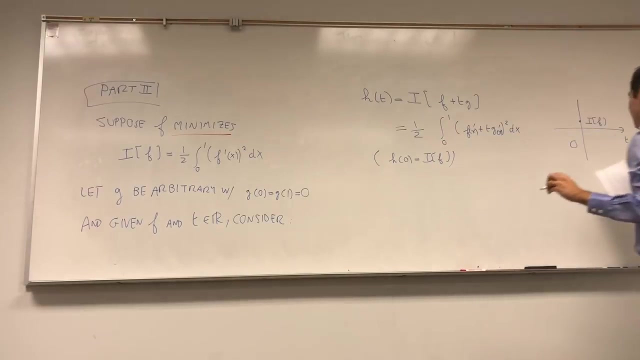 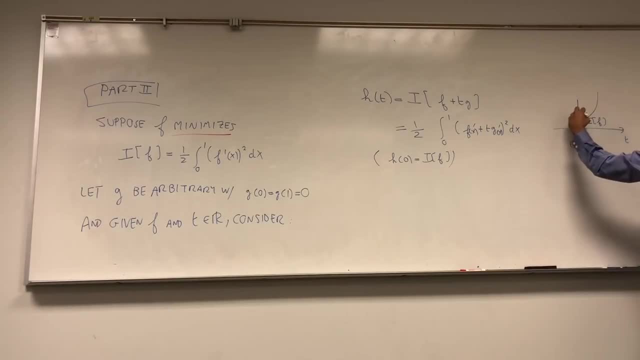 Okay, Yeah, Okay, Okay, Okay, Yeah, Okay, Yeah, Yeah. So that means that any other value of t that you pick, it cannot be the smallest one. At least locally, it can't be the smallest one. 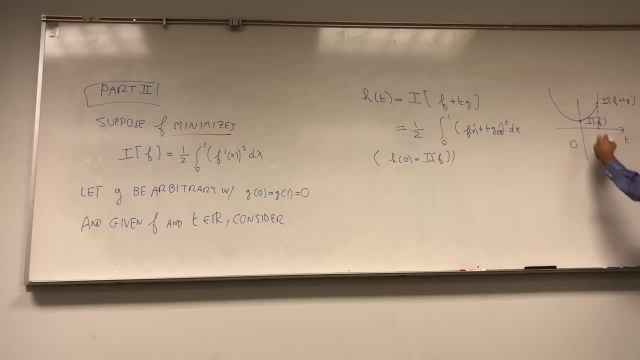 So if you pick another value here- i of f plus tg, Because f minimizes this, I mean it's possible that it's equal, but like it can never be smaller, if you want. So, In particular, if you look at this picture and let's say this is h of 0 and h of t. 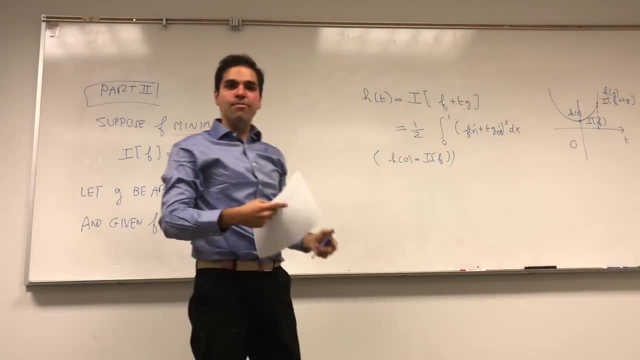 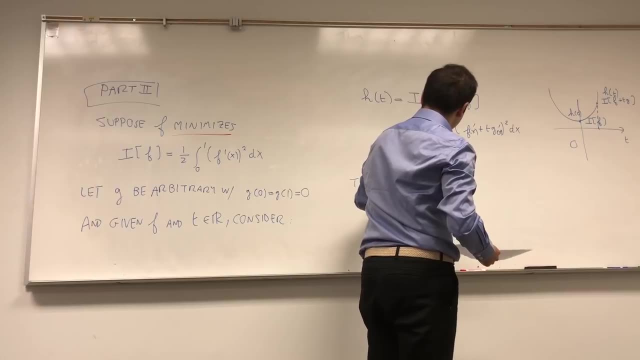 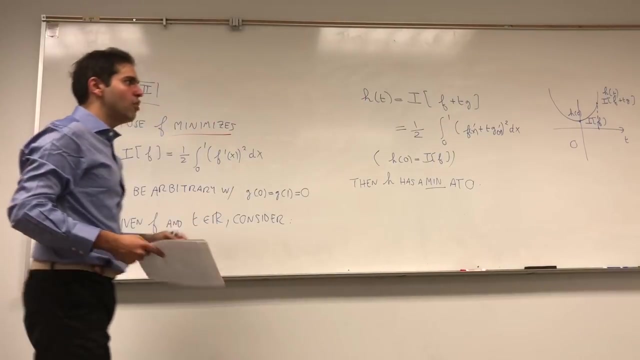 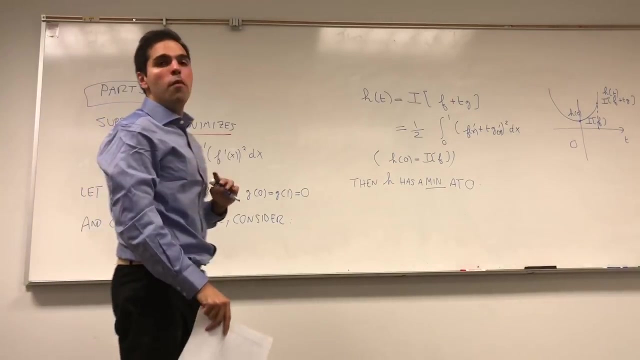 we can say for sure that h has a minimum at 0. That h has a minimum at 0. Again, because i of f is the smallest value. And now here's where the calculus comes in. What do you know about functions which have a minimum at the number? 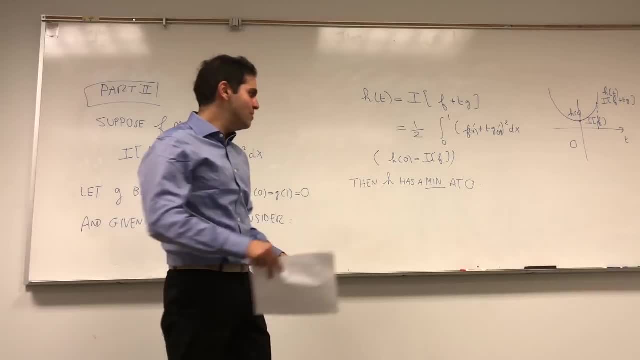 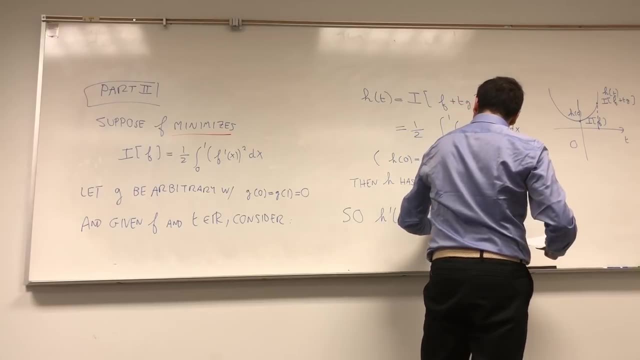 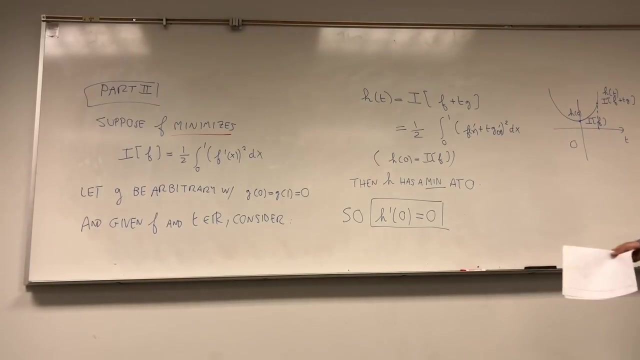 Well, it means their derivative is 0. It has to be a critical point. So h prime at 0 equals to 0. And this, precisely, is the passage from function spaces to single variable calculus, Thanks. So now that we have this info, let's calculate h prime of t. 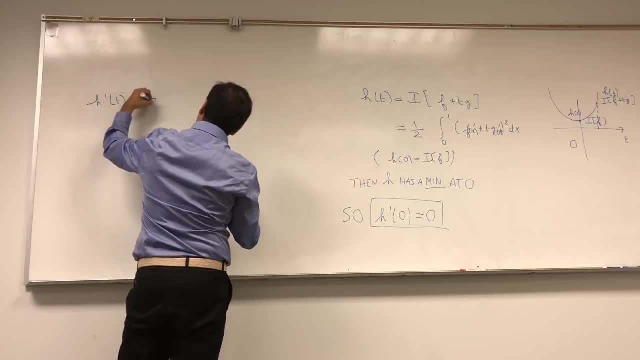 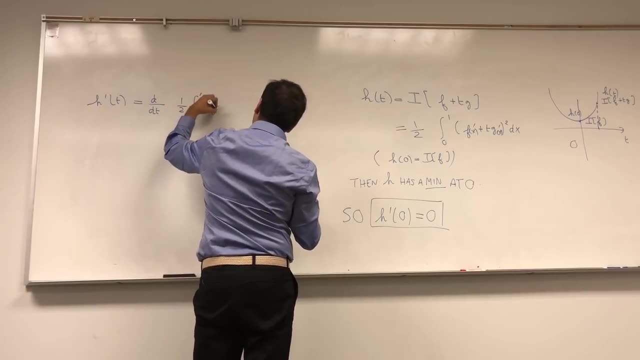 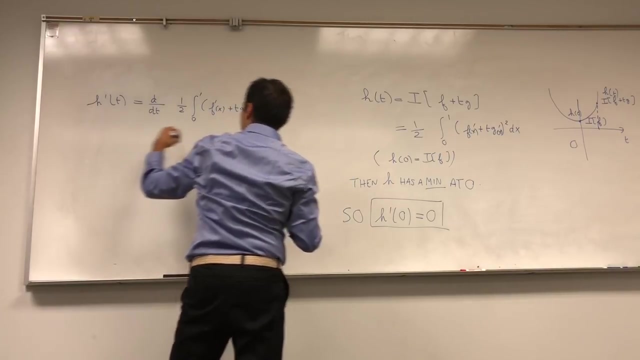 h prime of t, that's d over dt. One half integral from 0 to 1 of f, prime of x plus t. g prime of x, squared dx. Again, stuff is smooth so we can just pull everything inside of the integral. 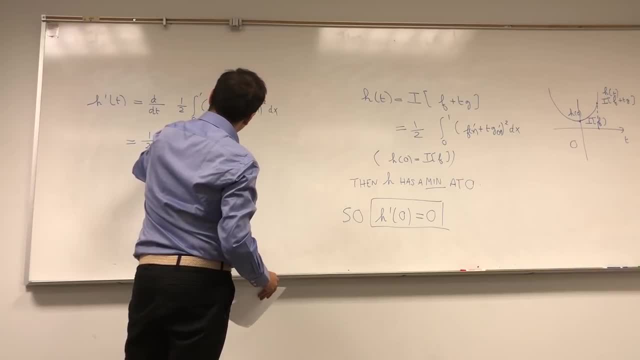 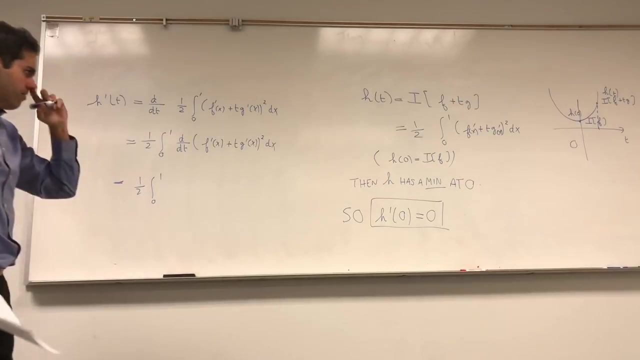 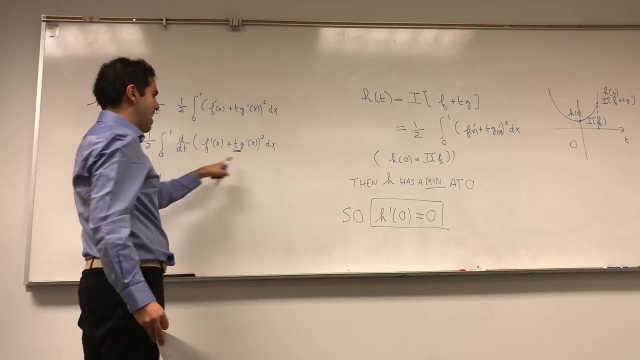 0, 1, d over dt, f prime of x plus t, g prime of x squared dx. And then let's just calculate that integral from 0 to 1.. And remember, this is a function of: we want to differentiate with respect to t and not with respect to x. 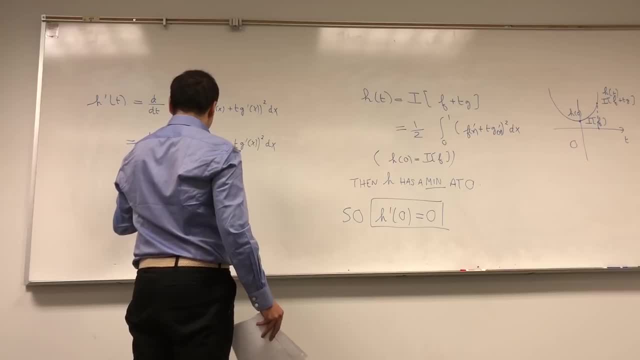 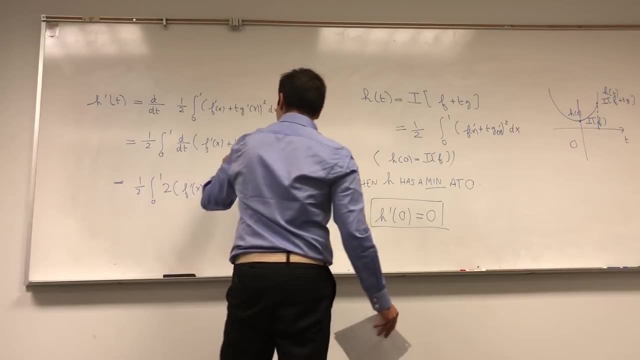 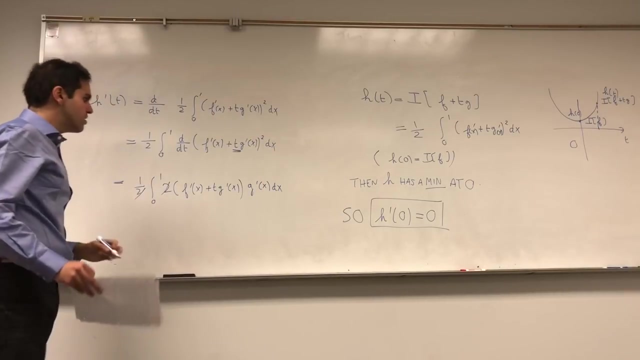 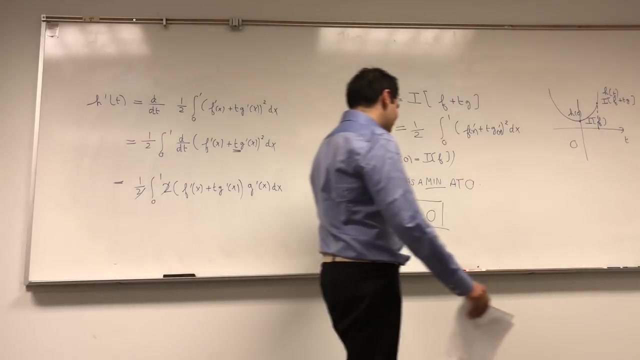 So there's no double prime here. So it's really 2 times f prime of x Plus t g prime of x And then times g prime of x, dx And the 2s cancel out And, as I said, we want to use eventually the fact that I've written down 10 minutes ago. 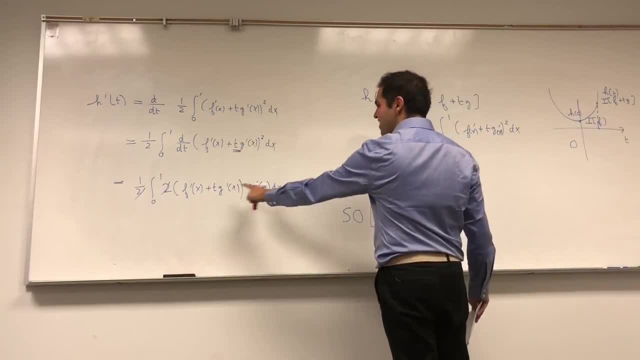 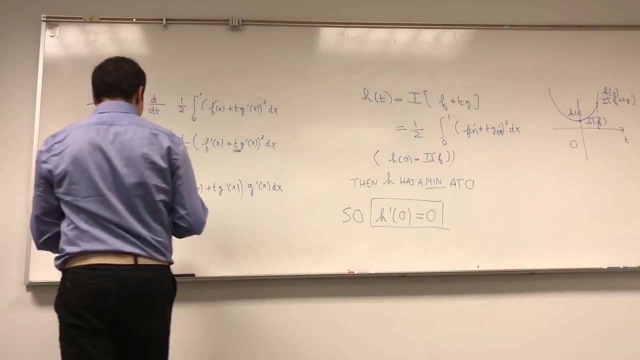 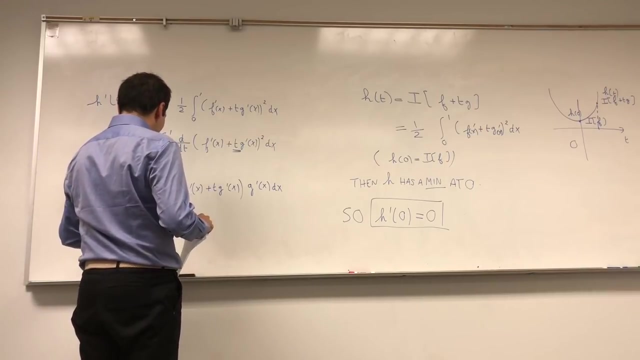 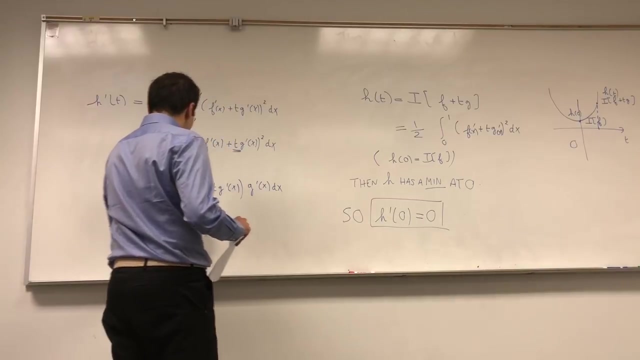 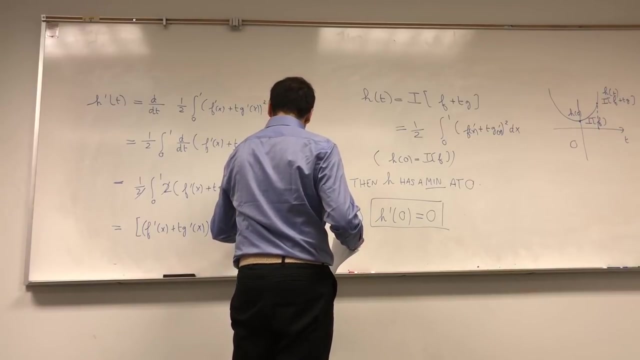 And if you think about this, this is actually a very nice, you know, job for Mr or Mrs: Integration by Parts. So let's integrate this by parts And again I'm getting, I'm making a point here. So that's really f prime of x plus t, g prime of x times g of x from 0 to 1, minus integral from 0 to 1.. 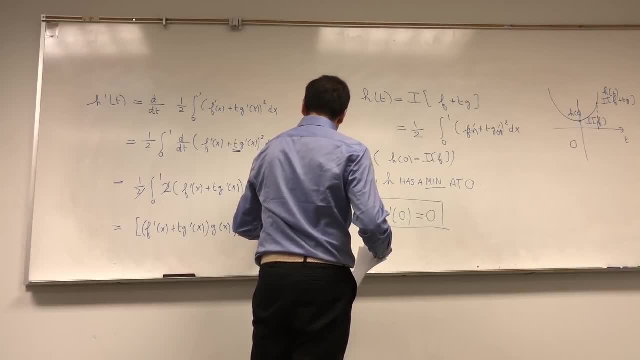 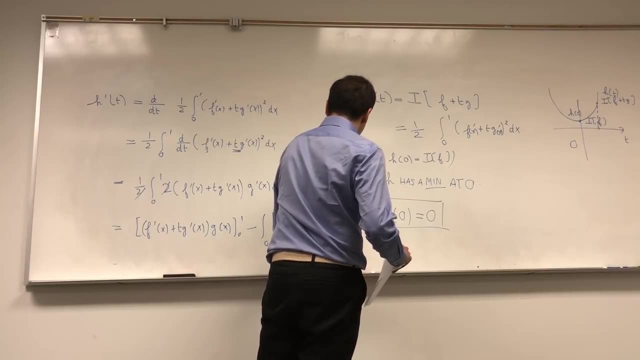 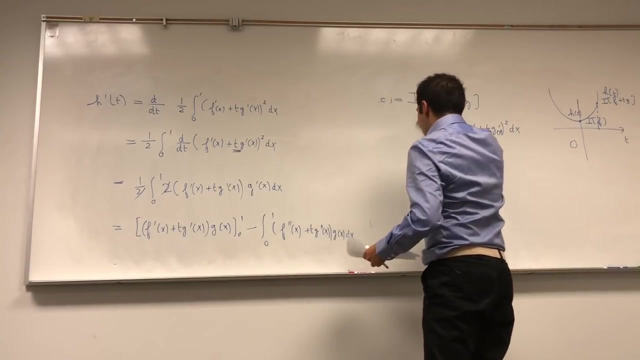 And now we put the derivatives on the x's: f, double prime of x plus t, G, double prime of X, G of X, the X. And here comes a cool thing: Remember what is G? It's a function that's zero at zero and one. 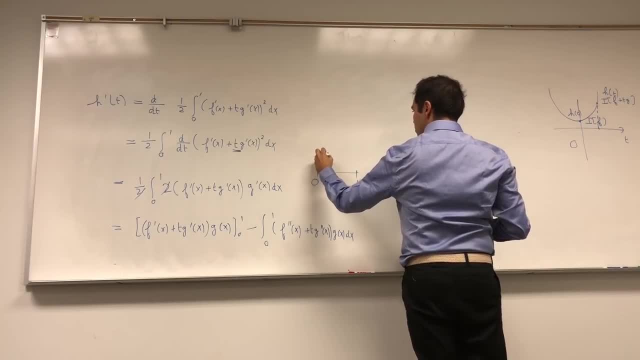 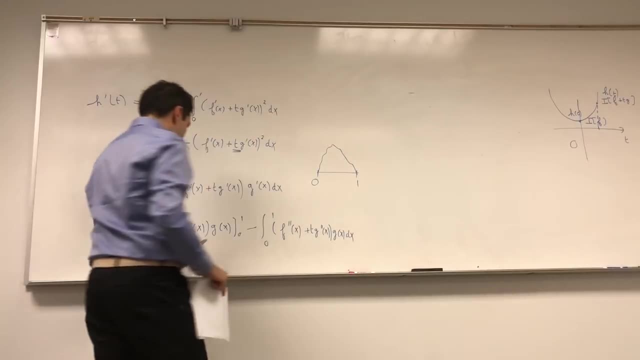 So it's zero here and zero here It could be. you know, imagine it's positive because it's for any G okay, And therefore, if you plug in one and zero, you get G of one and G of zero, which gives you zero. 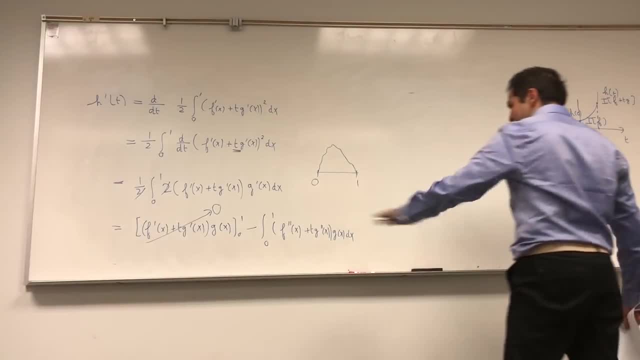 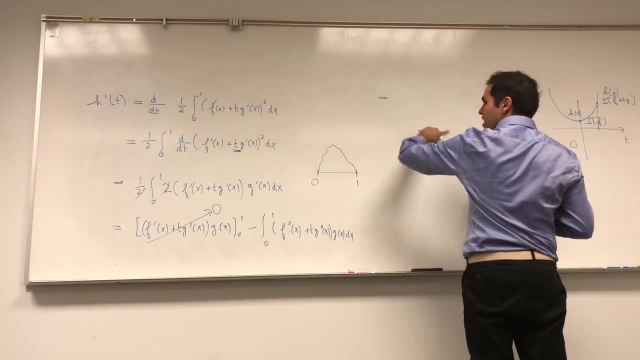 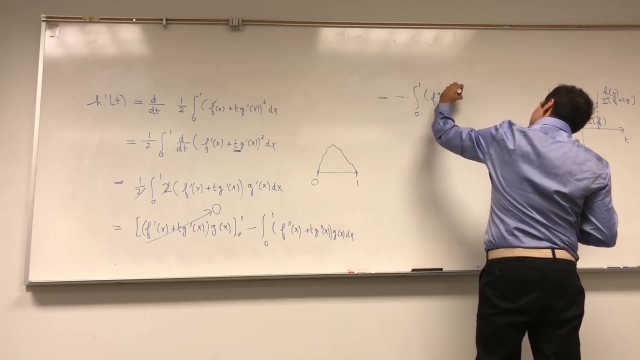 So in fact we chose a function G such that there is no end points. right, It's zero at the end points. So in the end the derivative of H of T becomes minus integral from zero to T. F, double prime of X plus T. 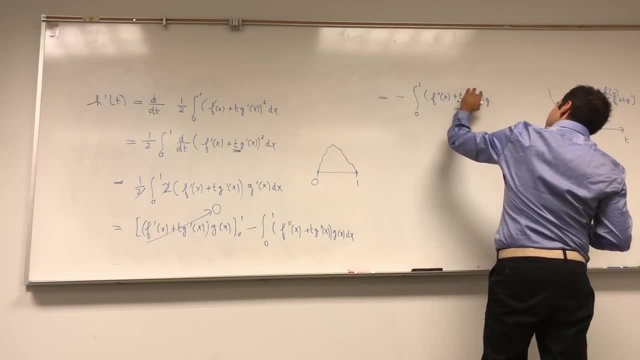 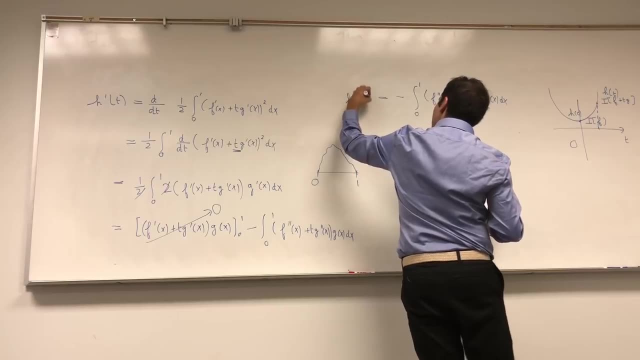 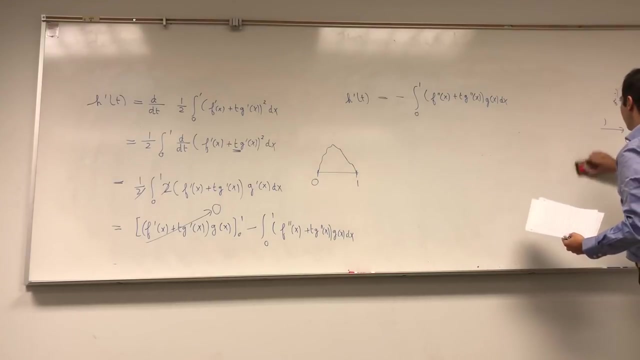 G double prime of X, G prime of X. sorry, G double prime of X, G of X, the X, that's H prime of T. And now remember, we know that H, prime of zero equals to zero. So let's just plug in: T equals to zero. 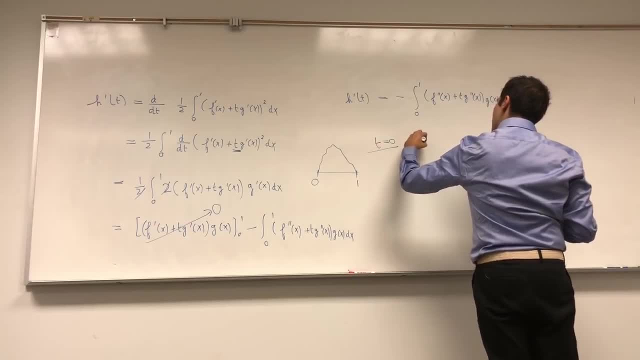 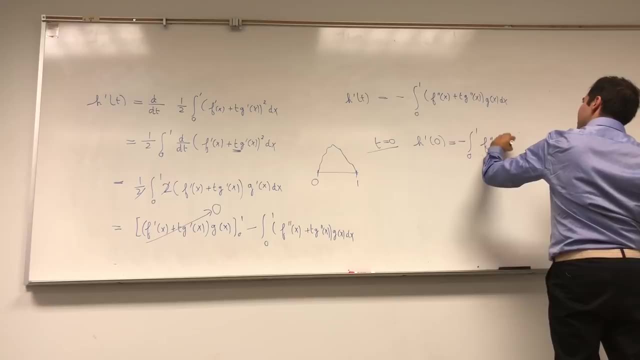 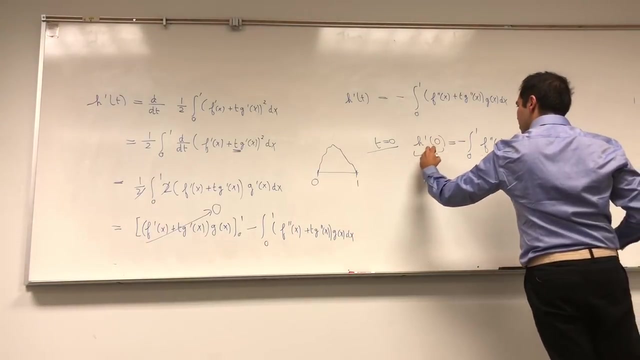 So T equals to zero. gives you H. prime of zero is minus integral from zero to one. F double prime of X, G of X, the X, And remember you know that this is zero. So what we get now is minus integral from zero to one. 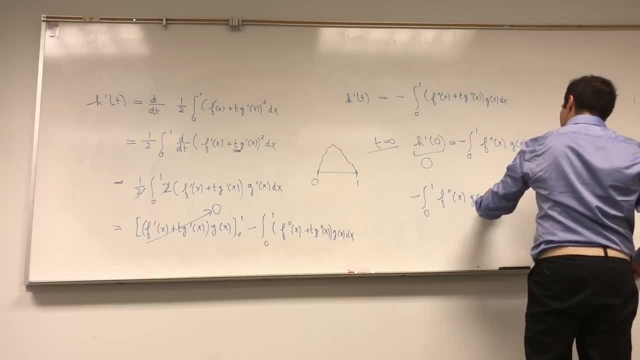 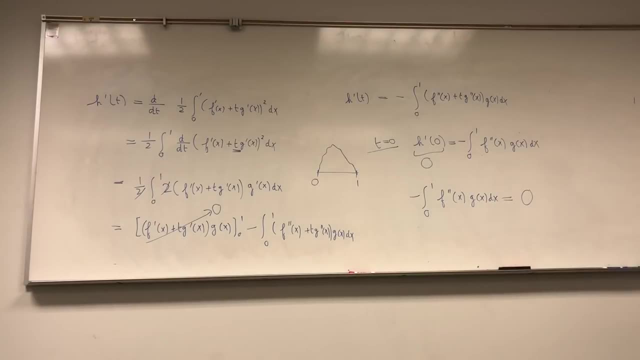 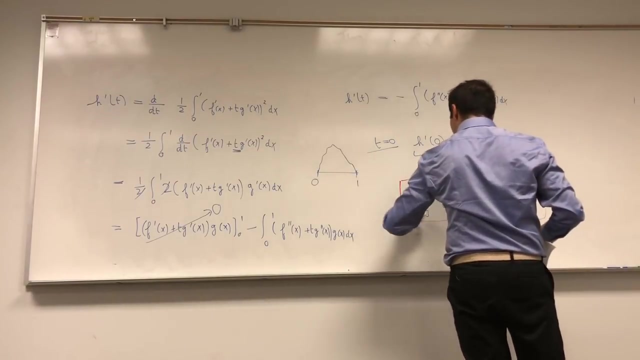 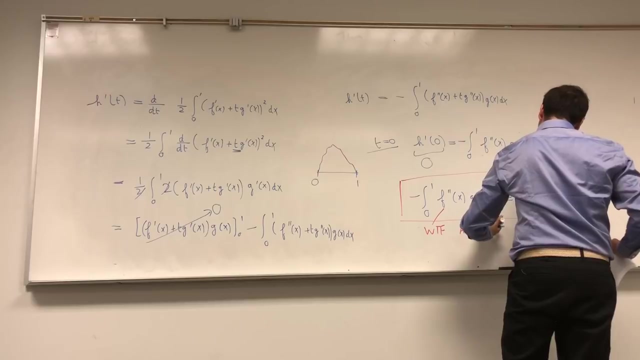 F, double prime of X, G of X. the X equals to zero. And here's an important thing, This is true for any function. G, right, Remember, we want to find F, F and this is arbitrary. So this is true for any G. 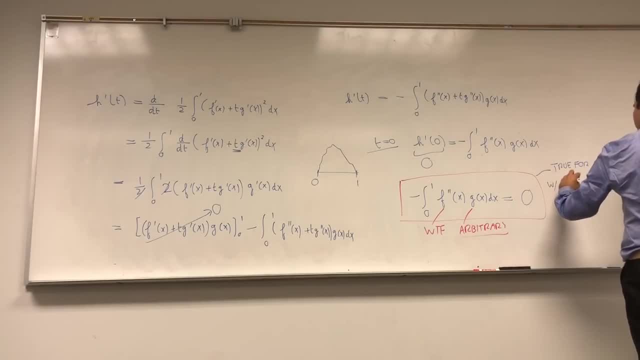 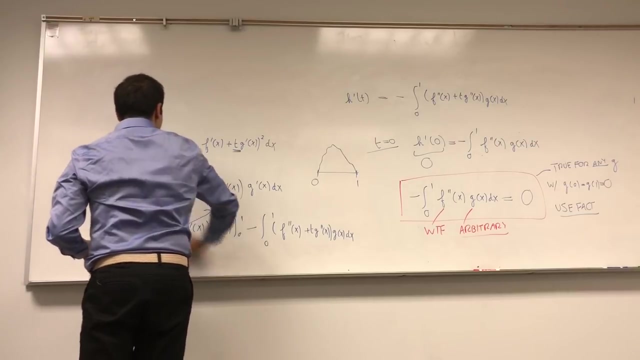 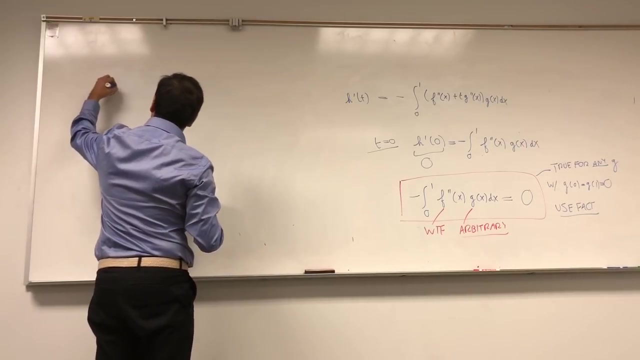 any G, in particular positive ones, with G of zero equals to G of one equals to zero. So by the fact, so use fact, what this fact says is that this function has to be precisely equal to zero. So so by the fact, 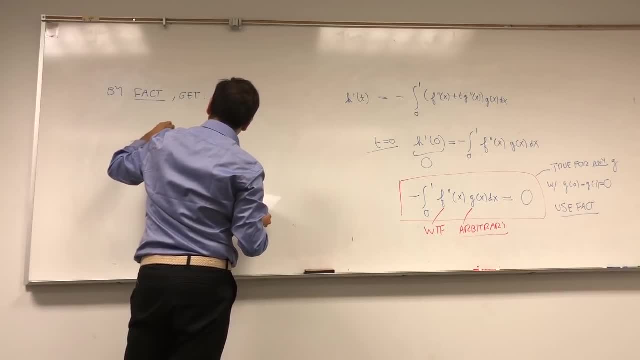 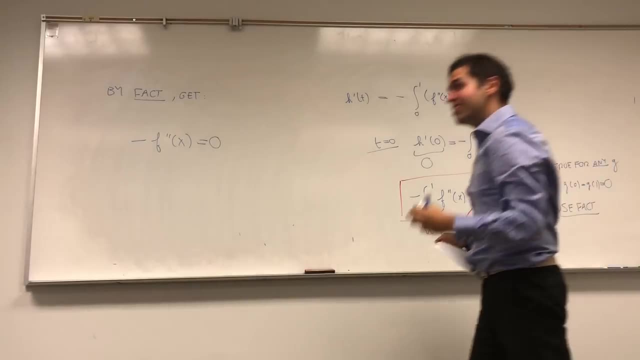 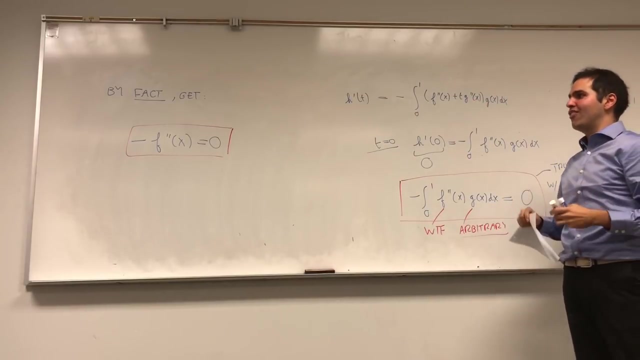 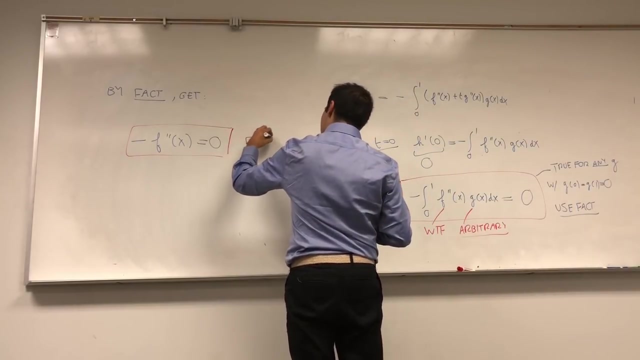 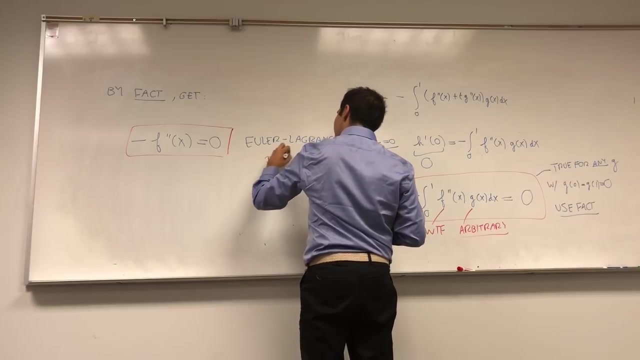 we get that minus F, double prime of X equals to zero. In other words, the solution of our minimization problem has to satisfy the following differential equation, which here in general it's called the Euler-Lagrange equation, In this case ODE, but in general it's a PDE: 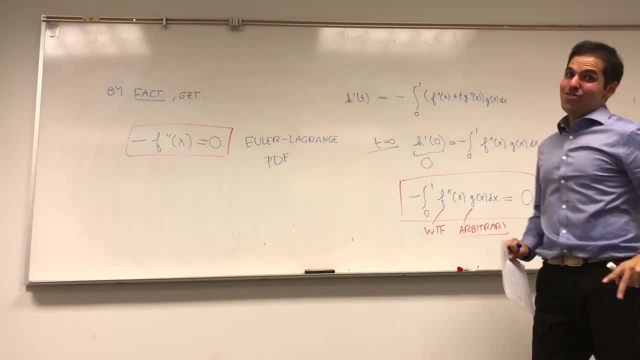 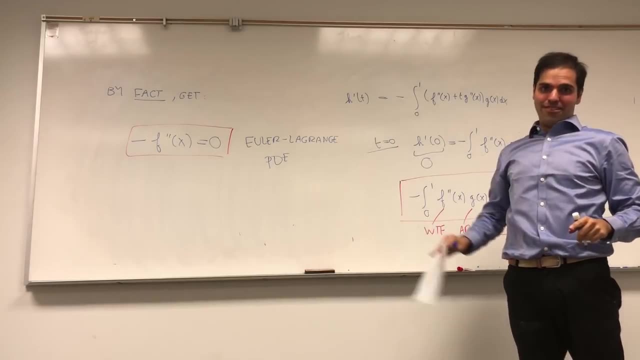 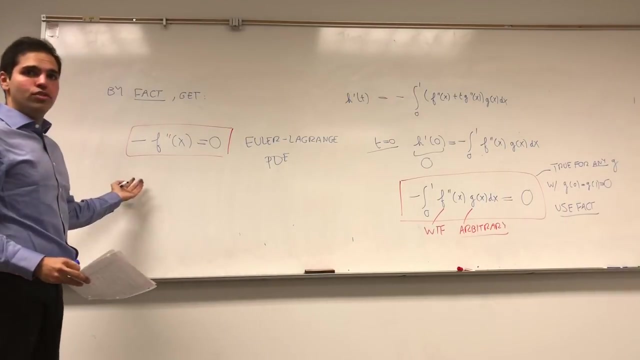 And notice Euler and Lagrange. they're two very important names, And if a theorem is named after really important people, it's very important. So it's a very important differential equation And in general it's hard to solve, but here it's not too bad. 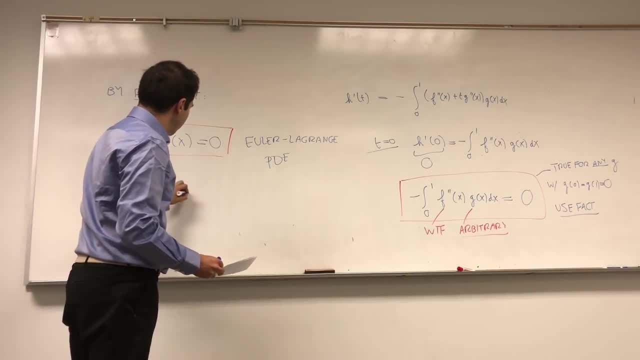 We get F of X If you anti-differentiate twice. it has to be a linear function. But remember: F of zero is zero And F of one equals to one, And the only function that satisfies this is F of X equals to X. 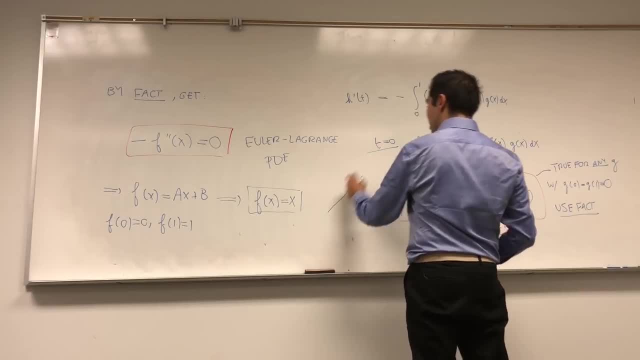 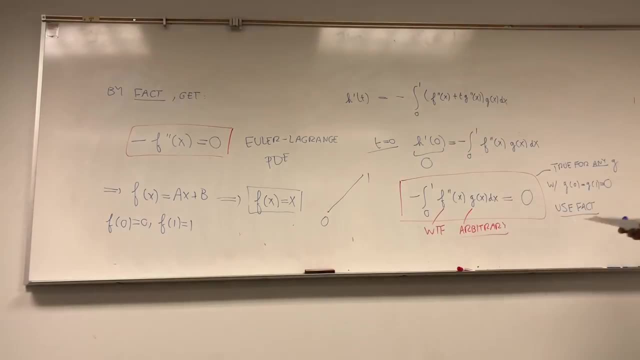 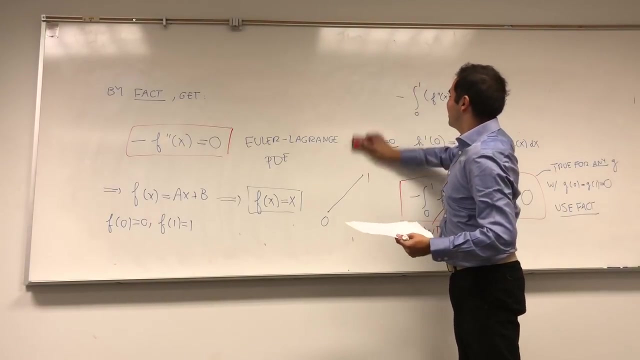 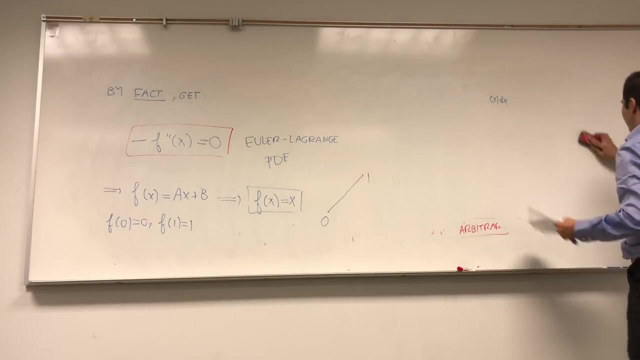 So, in particular, if your function is smooth and it minimizes the energy, then it has to be the linear function. But just a little bit careful, because we assume that F is differentiable. but it turns out, and this is, I think, a very nice research field- 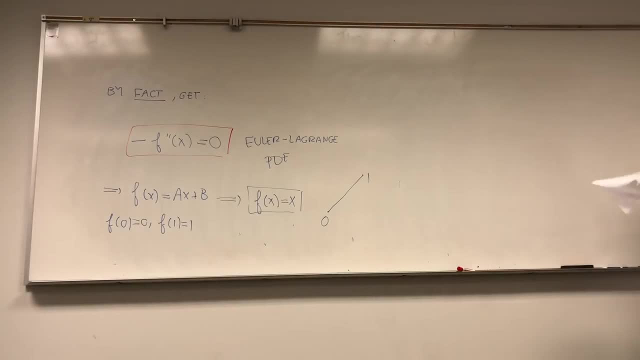 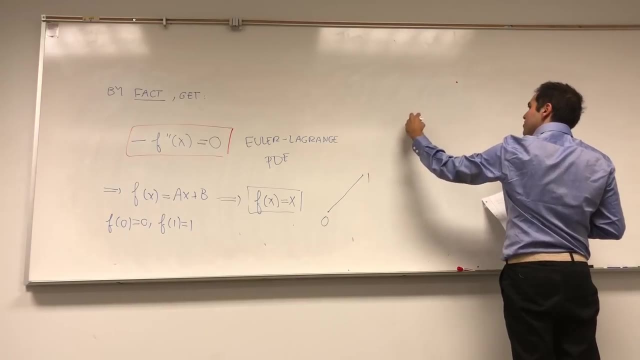 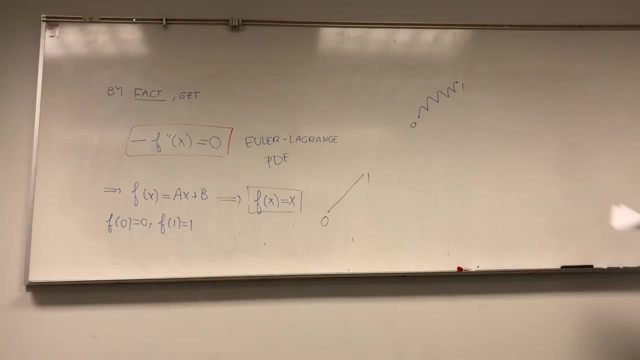 is to find non-differentiable solutions to this, And in fact, for example, this zigzag function here from zero to one. it actually also satisfies this what's called this energy. It's also another minimizer of the energy. 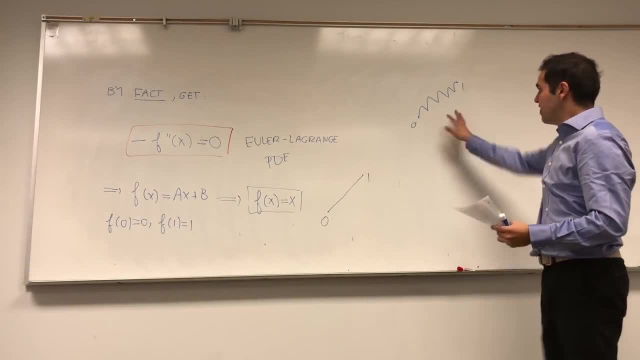 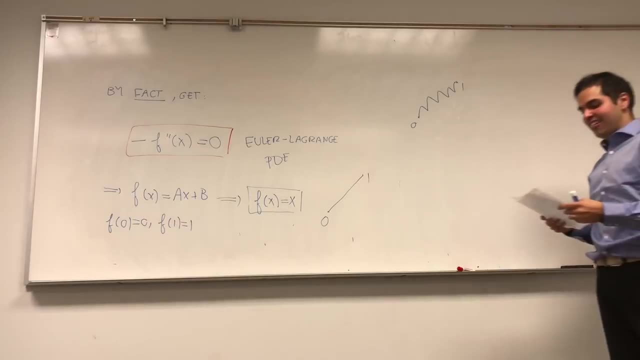 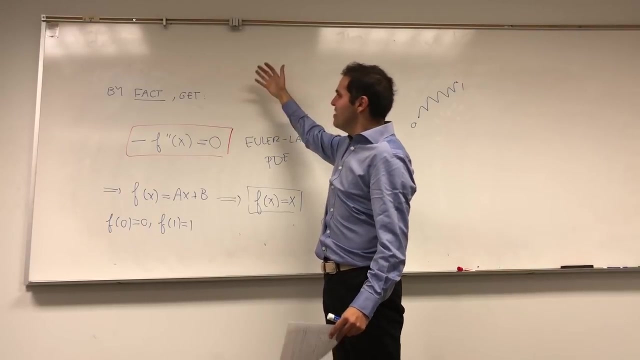 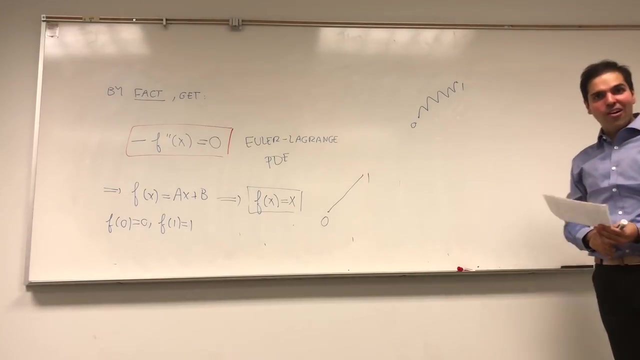 which is super exciting because in this sense, you can find non-differentiable solutions to this, So you have more generalized solutions. Again, the exciting thing was we took this minimization problem and turned it into a differential equation And, in fact, for the last part, 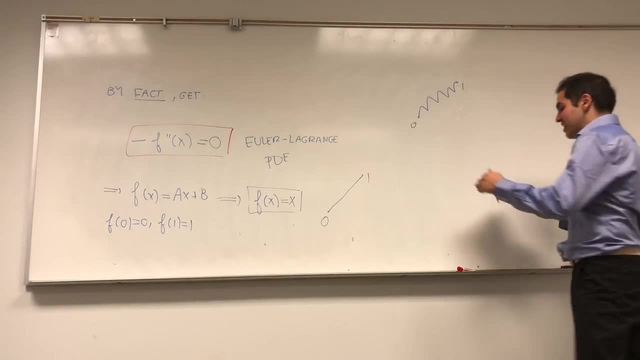 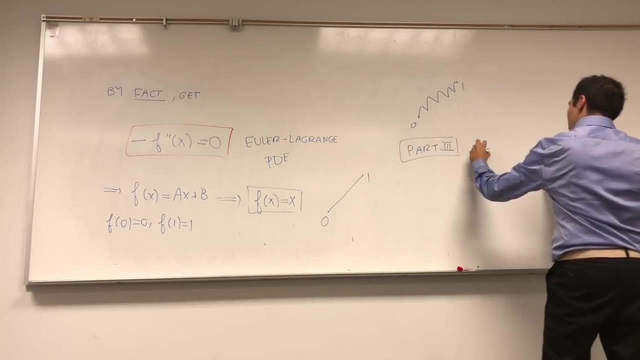 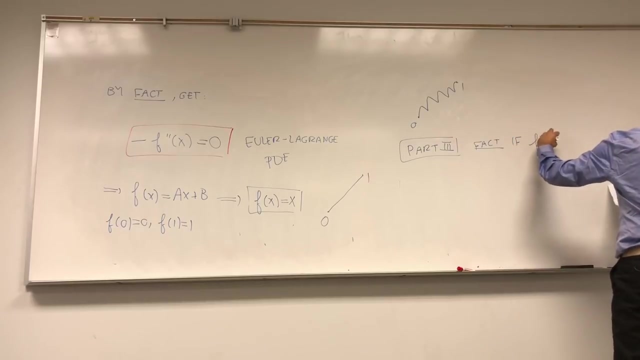 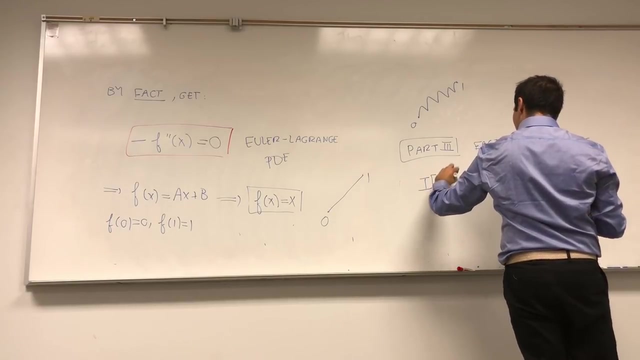 I just want to show you you can generalize this to higher dimensions. So part three. So suppose here's a little fact. if F minimizes the following differential, the following: functional I of F, which is one half integral of U, 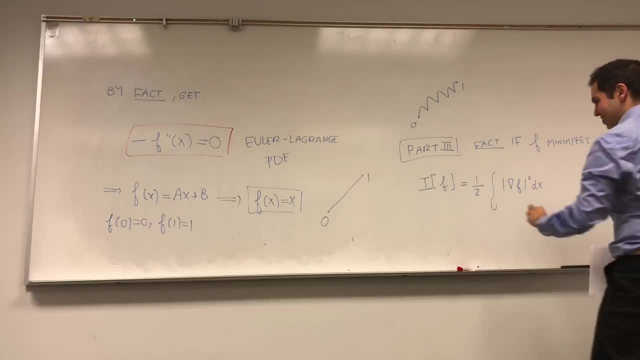 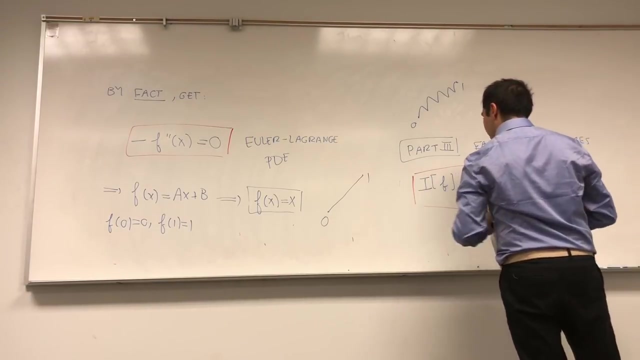 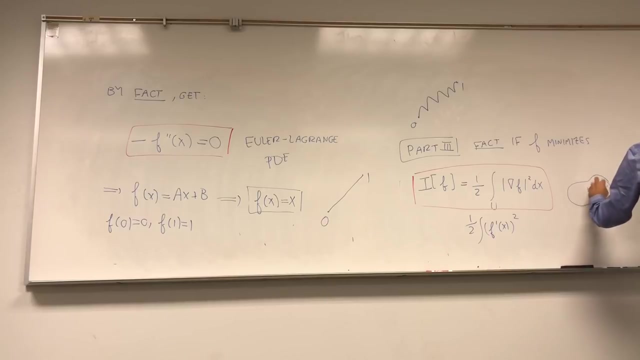 the gradient square of the X. So compare this with one half integral of F prime of X squared, Literally the- you know, n-dimensional analog of this. And U is an open bounded subset, So U is open bounded in Rn. 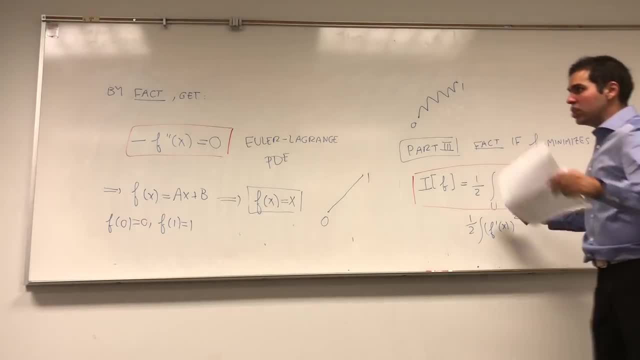 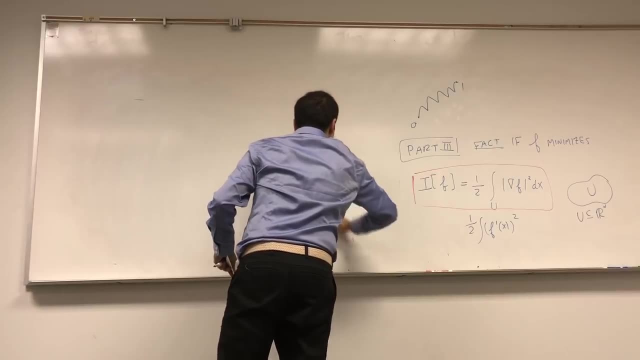 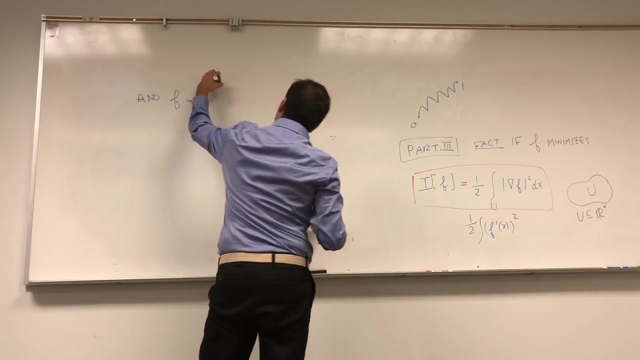 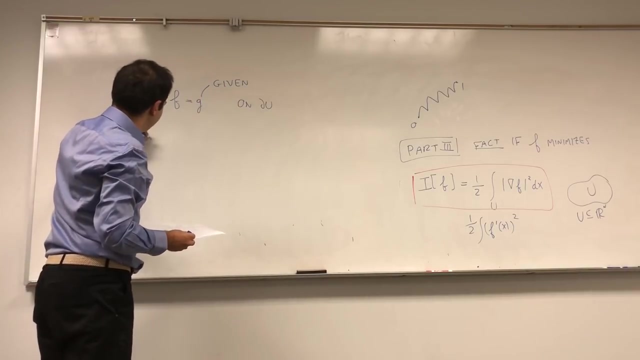 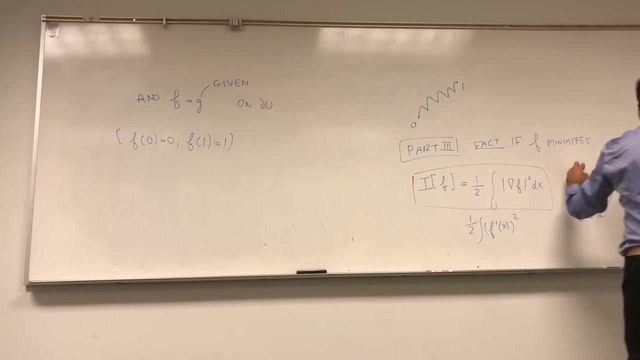 And suppose that F is equal to some given function on the boundary And F equals to G given on the boundary. This is, if you want, the analog of F of zero equals to zero, F of one equals to one. So if you have your set here, 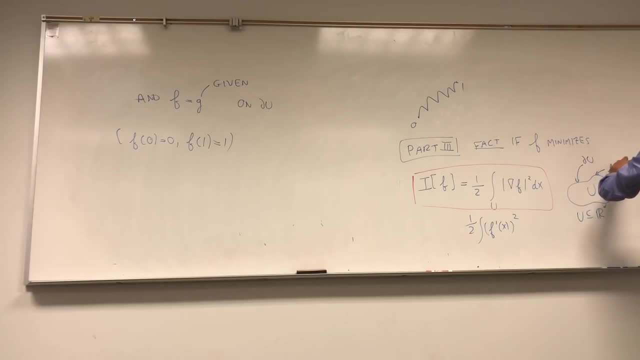 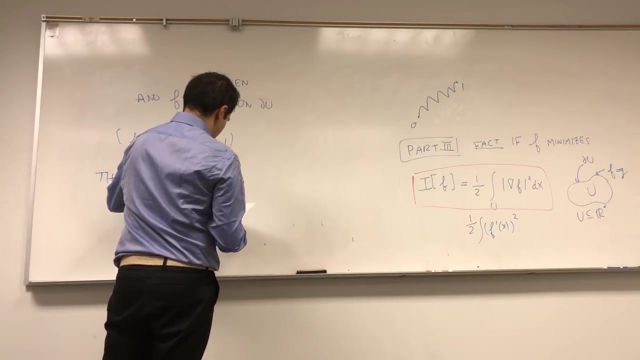 and you have a boundary and you impose that F equals to G some given function. then F turns out to solve a very important PDE, namely Laplace's equation. So then F solves minus Laplacian of F equals to zero in your set. 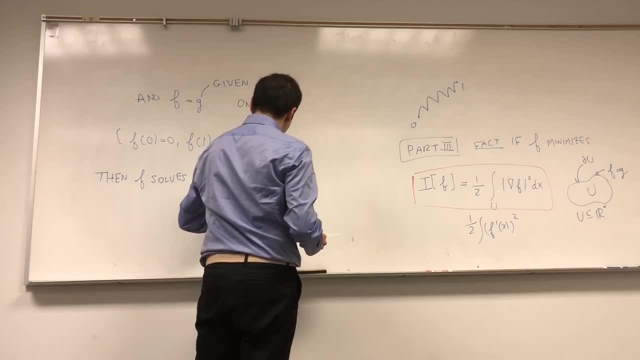 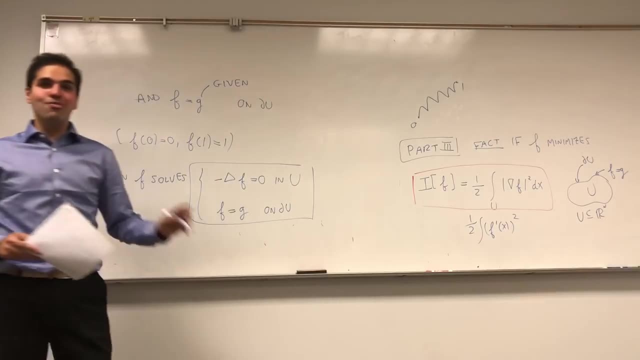 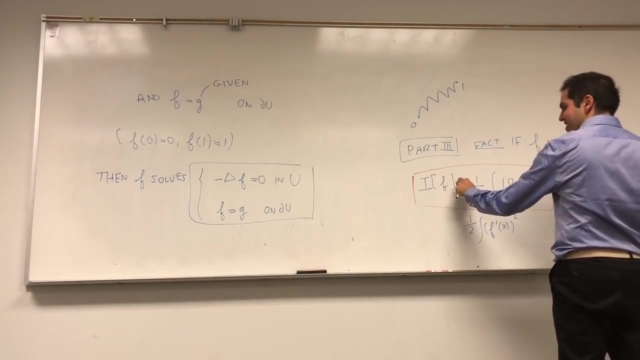 and F equals to G on the boundary And, surprisingly, the proof is exactly the same, Namely, you just pick some other function, you know, I guess G, or not quite G, but like G squiggle, and you consider H to be I of F plus TG. 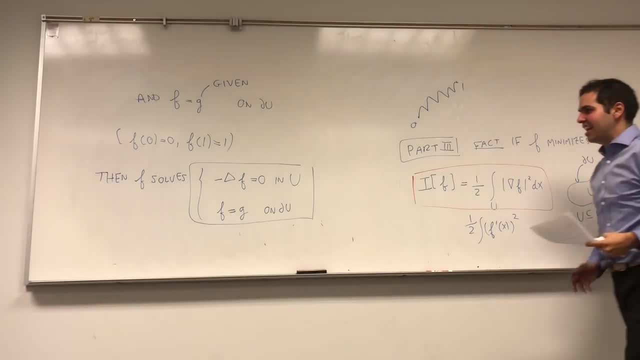 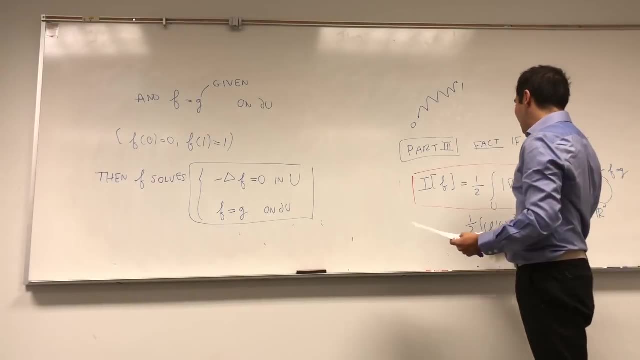 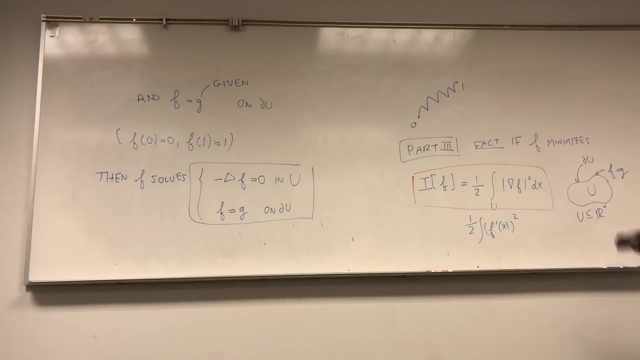 and then you do the same thing where you differentiate, and in the end you get this Laplace's equation, which again helps us find solutions to Laplace's equation. just find minimizers of this functional. And you might also ask: 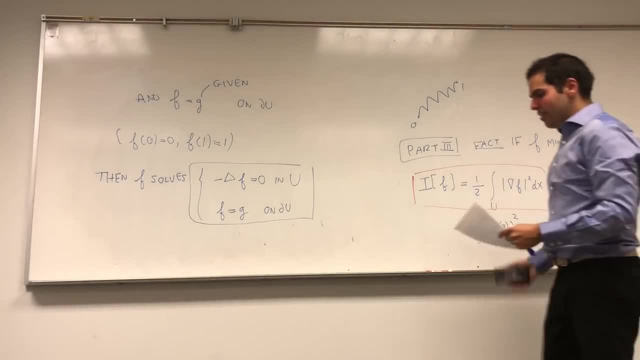 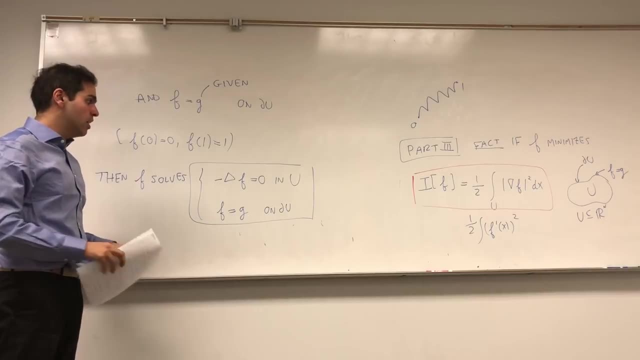 why in the world this is important? because here we're lucky, because it turns out we can solve Laplace's equation, not a problem at all. but sometimes your PDEs are extremely hard to solve and there's no way to even get a formula. 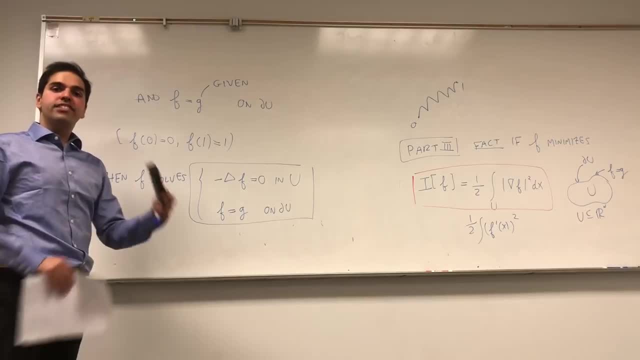 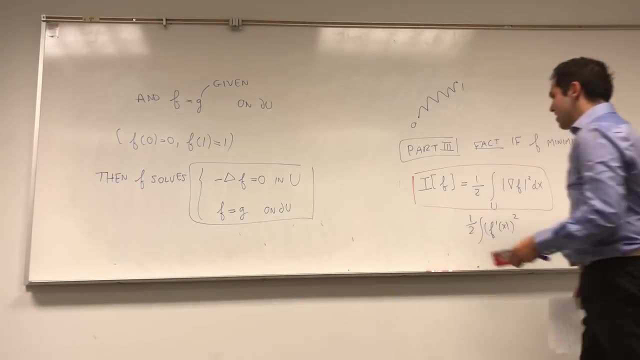 with this. Well, if somehow you can say that this has to be a minimizer for some energy, then sometimes it's easier to find the minimizers of energies And once you have that, maybe you have hope of finding solutions to your PDEs. 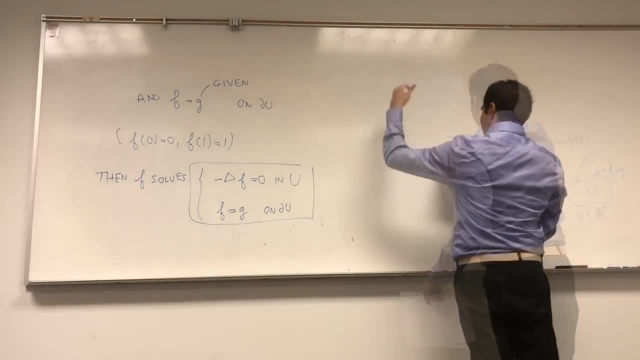 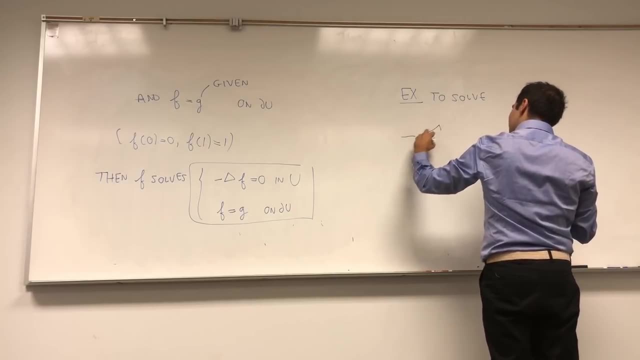 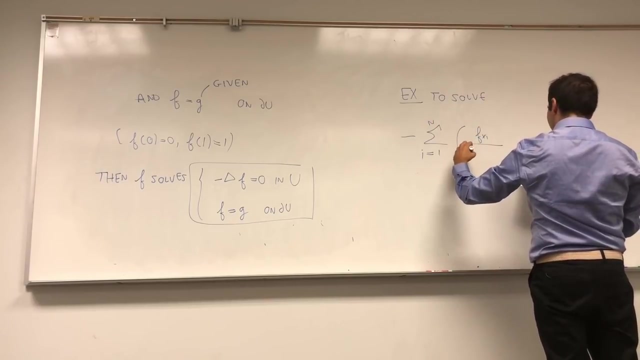 Let me give you a specific example. What does he want to solve this? Okay, To solve the following equation: sum from 1 to n of f of the i-th derivative of f, plus 1, plus gradient f squared, and you differentiate that. 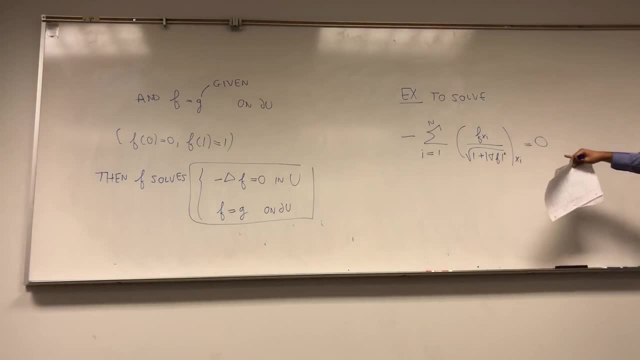 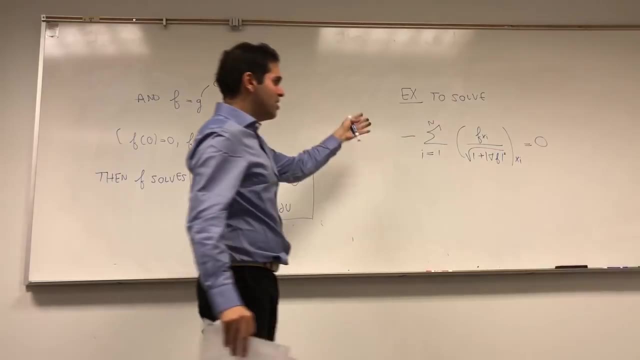 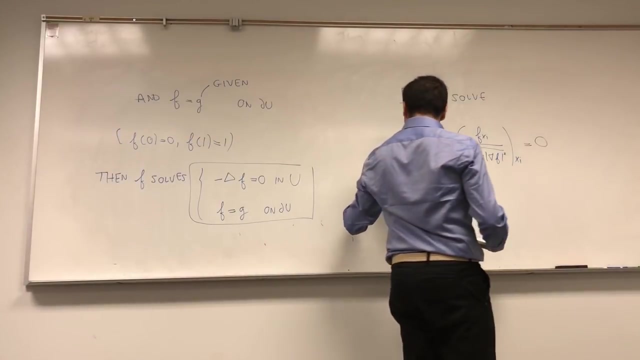 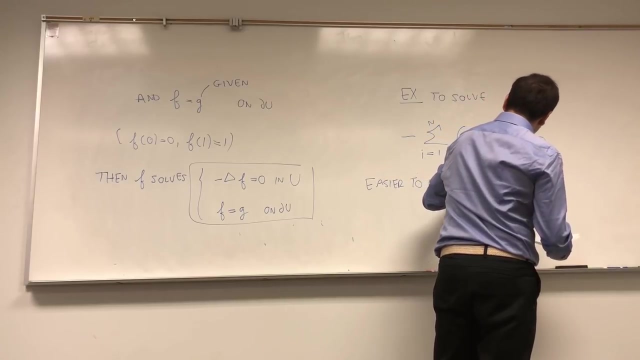 with respect to xi. Good luck solving that. You know it's a very difficult PDE. It turns out this becomes- you can write this equation as the minimizer of some- much easier, functional, easier to minimize the following one: i of f is. 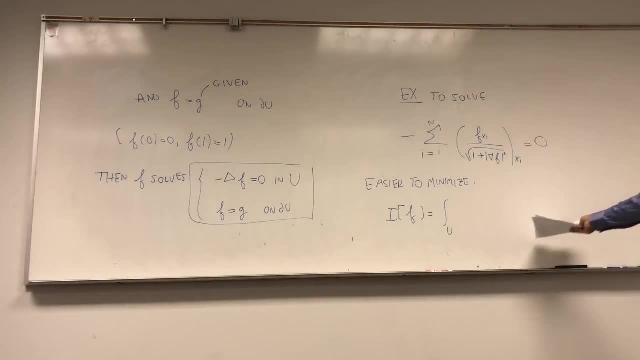 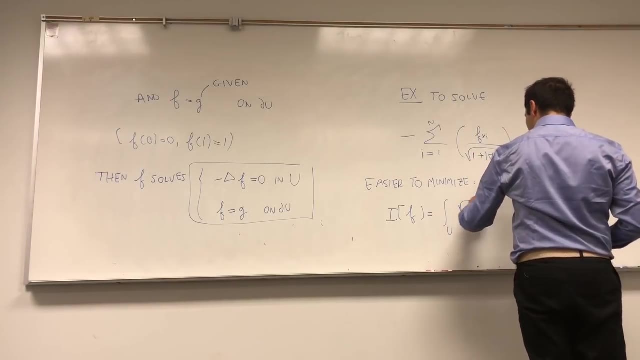 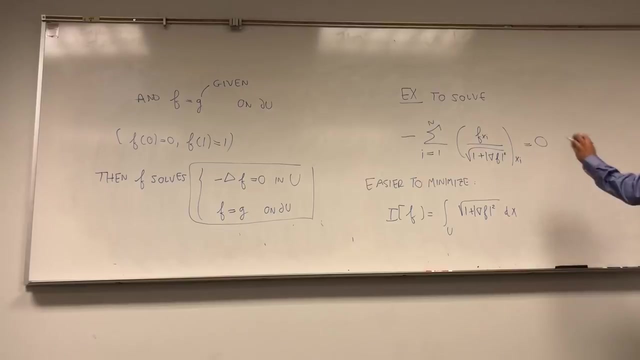 again. it turns out if you take the following minimizer and you find the Euler-Lagrange equation, the functional is just the following: 1 plus gradient of f squared dx, And if you remember your multivariable calculus, you may recognize this as. 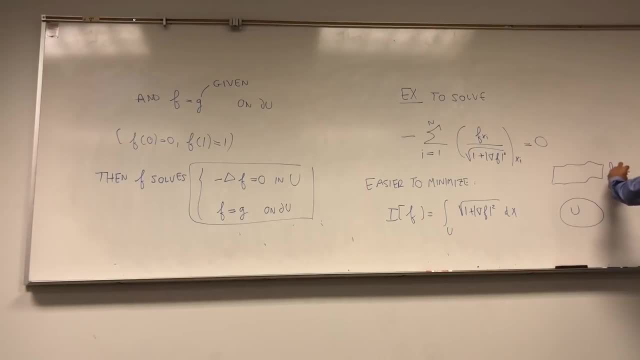 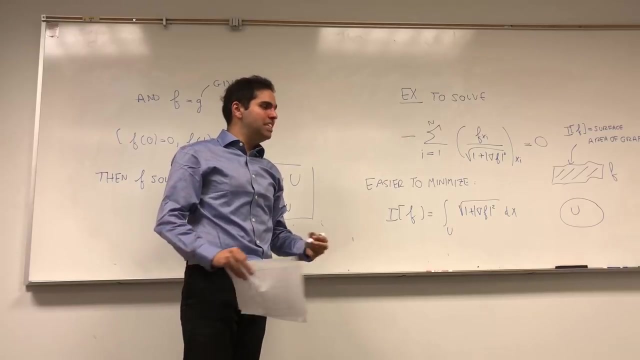 simply the surface area of the graph of f. So if you have some graph of f and you find the surface area, then i of f gives you the surface area of f of the graph. So instead of asking which functions solve this PDE. 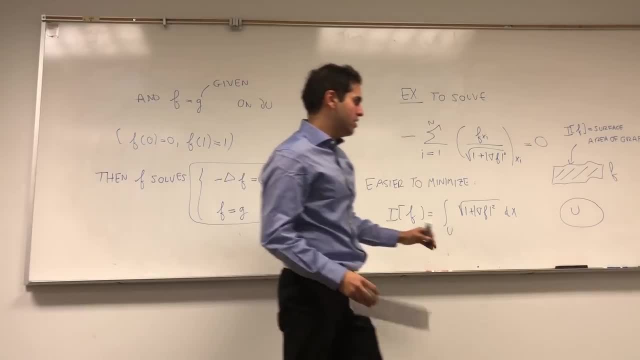 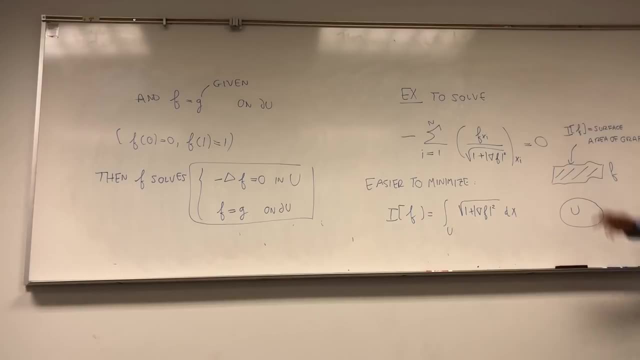 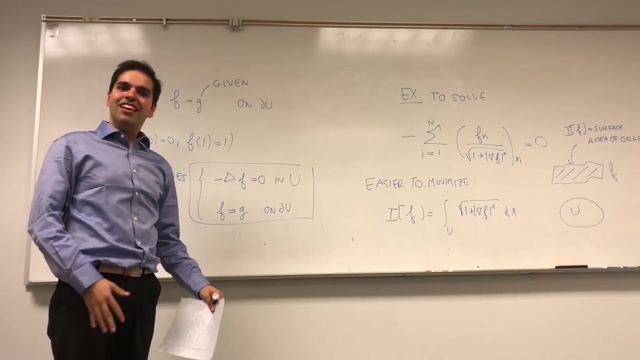 it's easier to ask- which functions, again with some boundary conditions, minimize the surface area of some graph, And this actually leads to a very beautiful subject of area-minimizing surfaces. And on the comment section or the description section I will put some very nice links.